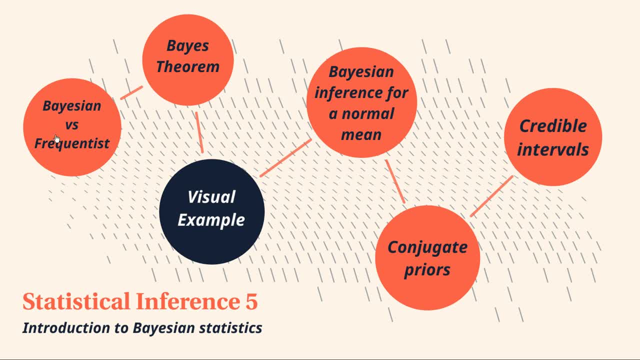 of Bayesian statistics adds something a little new. Well, in fact, it actually adds a different frame of reference, as we'll see, to the frequentist paradigm. We're then going to look at Bayes' theorem itself, which you learn when you do sort of. 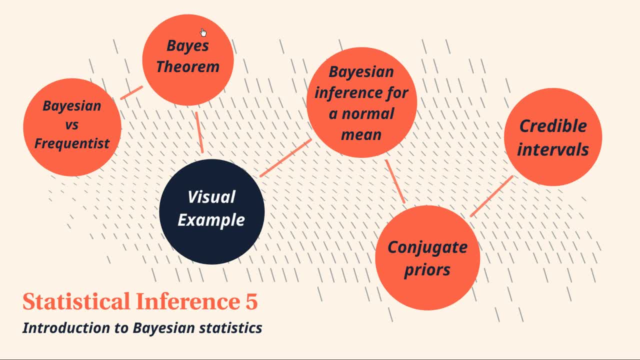 what Year 9, year 8, year 9 mathematics? maybe It's high school, So it's not a very complicated theorem, but its application to statistics is quite profound. So after we have those two under our belts, we'll have a look at a really cool visual. 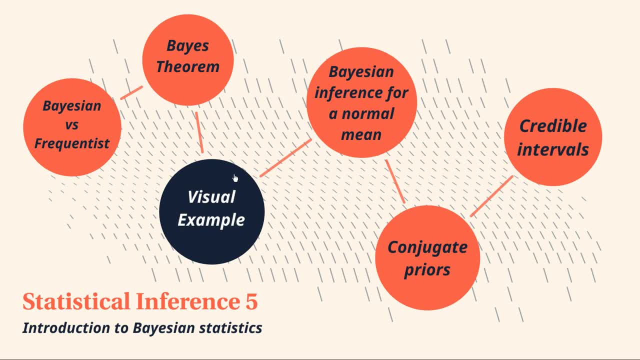 example, And this is where it all kind of connected for me when I first saw this particular example. So hopefully you'll stick with me until then, because I think that's a really good way of trying to get in your head an intuitive sense of how Bayesian stats works. 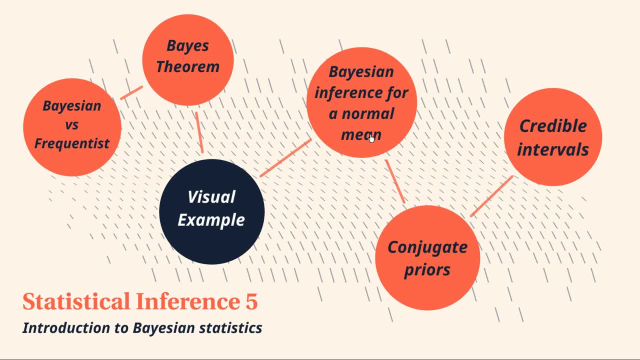 Okay, We'll then apply Bayesian statistics to a normal mean, a distribution for a normal mean or mean from a normal distribution. We'll then look at two particular subtopics around Bayesian stats. One's to do with conjugate priors And finally, we'll look at credible 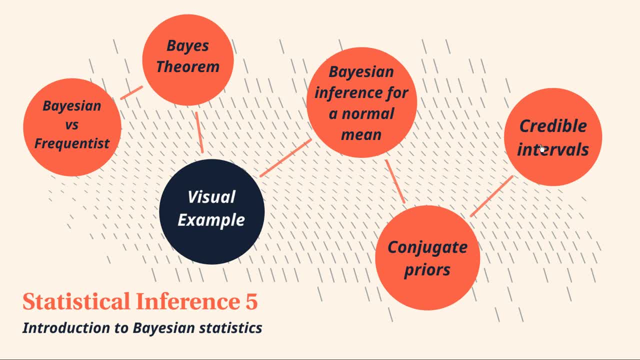 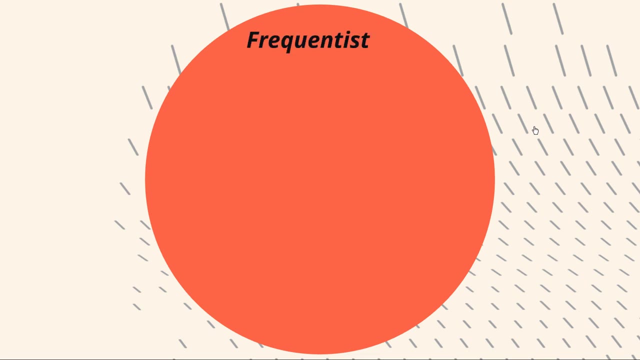 intervals, which are the Bayesian equivalent for confidence intervals. So let's start now by having a look at the differences between Bayesian and frequentist statistics, And we're going to start with frequentist, just to kick us off in a direction we're familiar with. 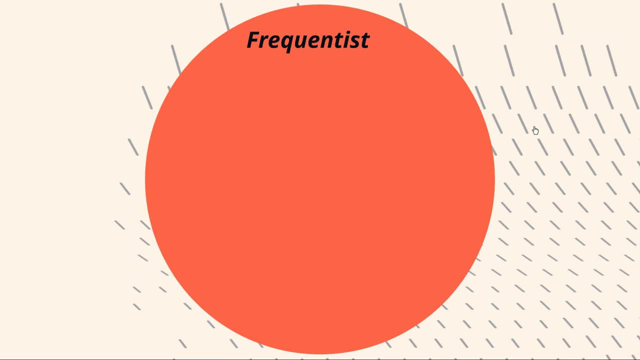 Now, in frequentist statistics, the focus is on the parameter And it's assumed to be a fixed constant. Now, if you've done any statistics before, you'll actually be familiar with this concept. We always treat the parameter as some kind of godly figure, right? It's unknown. 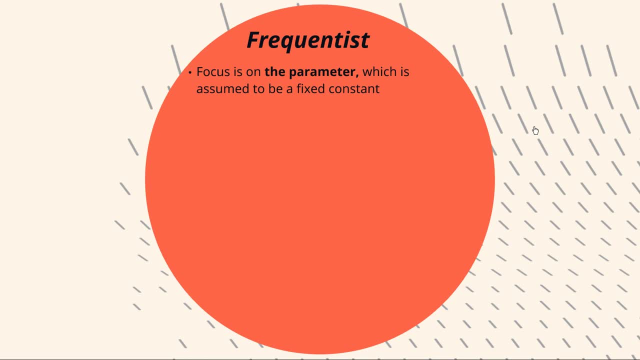 but it's always fixed and we try to do our best to estimate it. So when we construct confidence intervals, we read them in terms of repeated sampling. So technically, the way to interpret a confidence interval would be to say that 95% of similar 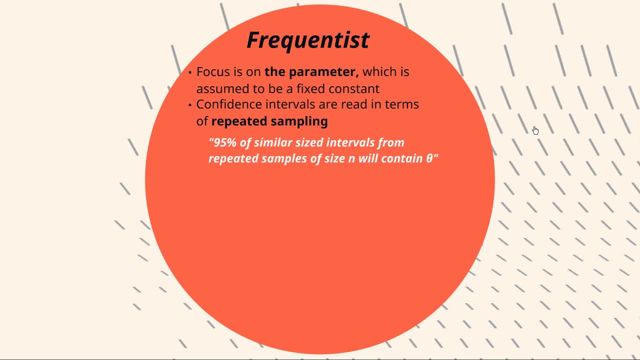 sized intervals from repeated samples of size n will contain theta, which is our population parameter. Now, as I said, that will probably be somewhat familiar to you, considering you've been conducting frequentist statistics Up until this point. But I might just re-emphasize the idea that it is about repeated sampling. 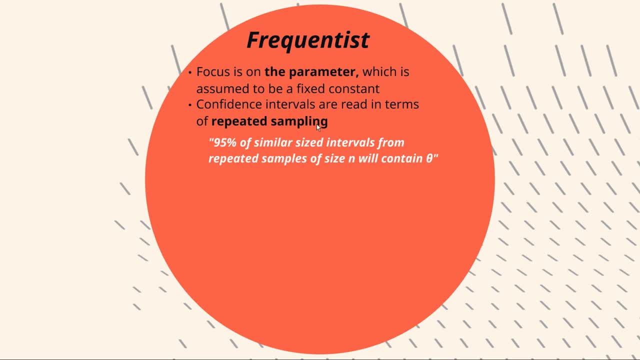 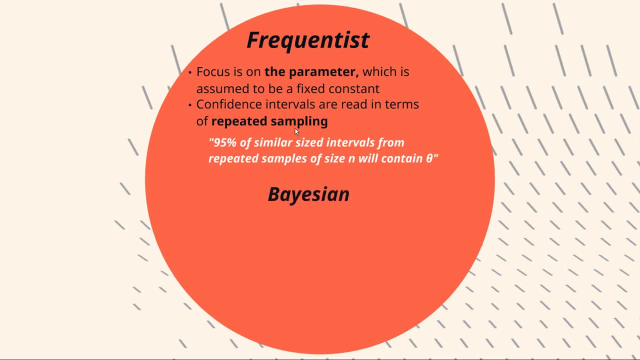 That's a frequentist approach. Why is Bayesian any different? Here, the focus is on subjective probability, meaning that we're looking at it from the perspective of the subject, the statistician, if you like. In other words, we're trying to assess the statistician's uncertainty and we also take into account her a priori. 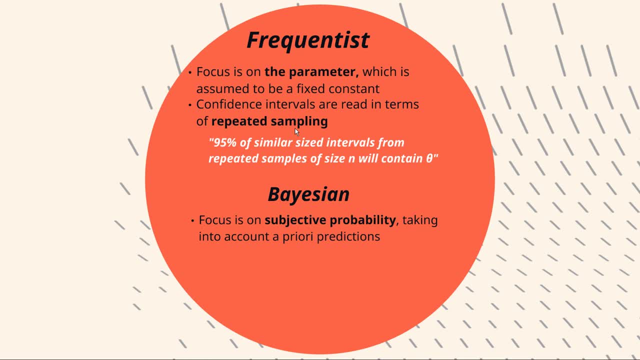 predictions. Not so interested here in whether the parameter is a fixed constant. All we're really focusing on is what the parameter is, and it's not particularly about the parameter itself. statistician can really know. So when we construct these things called credible intervals, which I 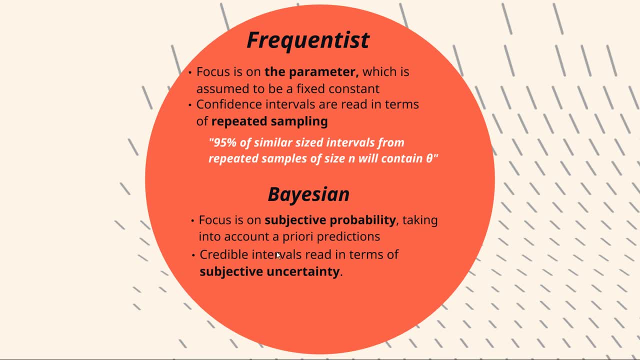 intimated before were the equivalent of confidence intervals. when we're dealing with Bayesian stats, we're going to read them in terms of subjective uncertainty, So the uncertainty of the person doing the stats right The subject. So it's all well and good to say that the parameter might be. 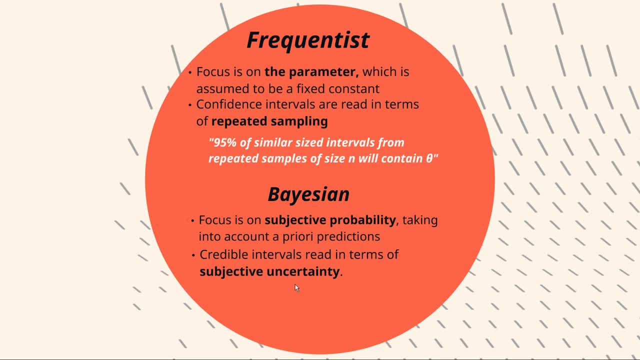 some fixed constant. but who really cares? It's me that's doing the statistics. So the parameter for all intents and purposes could be considered a variable from my perspective. So we can say that when we construct these credible intervals, there's a 95% chance that. 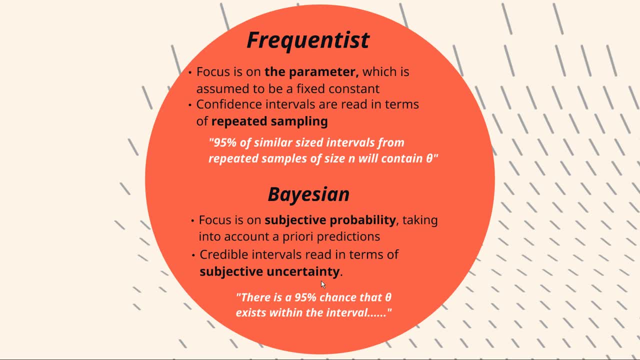 theta exists within that interval, which is actually a much more convenient interpretation. So that's really the allure of Bayesian statistics. You get these really nice interpretations where you can say, well, I'm going to do this, I'm going to do that, I'm going to do that, I'm going to do that. 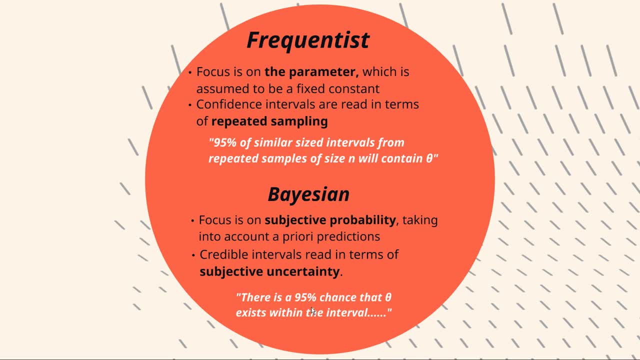 When you're dealing with uncertainty, And also there's quite a bit of power in taking into account my a priori predictions or my predictions about the parameter before we've even conducted the experiment. Now, if that still sounds a little bit airy-fairy for you, bear with me, because we'll. 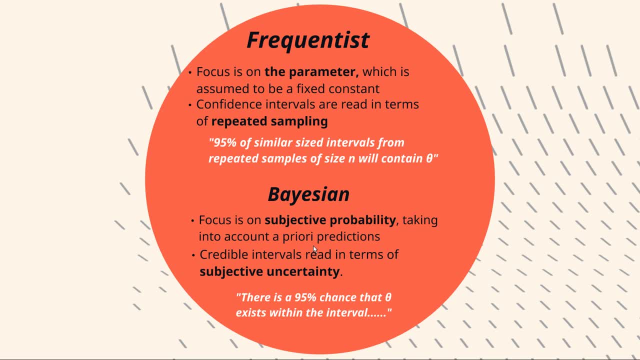 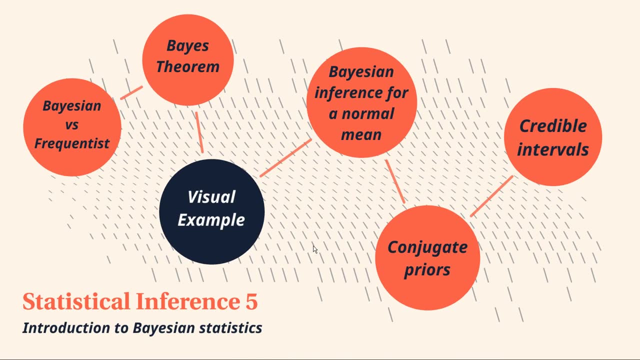 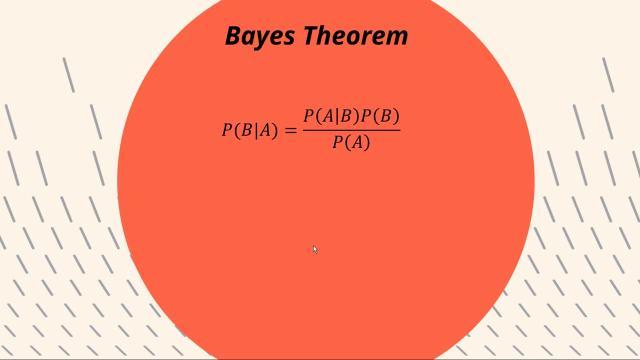 look at the Bayesian theorem itself and then we're going to do a little example where it will all hopefully come together for you. So let's do that now. Let's have a look at Bayes' theorem. So what does Bayes' theorem actually tell you? This is the formula that you get given. 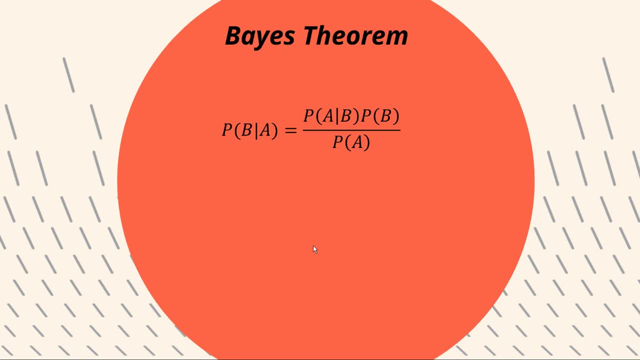 as I said, in what year 9 mathematics, maybe year 10 or something like that, where it says the probability of B given A is some function of the probability of A given B. So it sort of switches that conditionality around, And you might see this often. 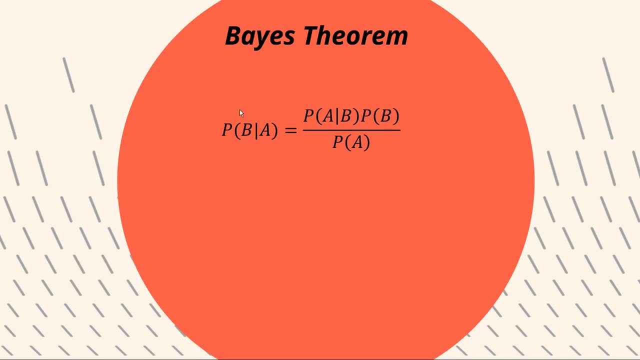 in biostatistics or statistics relating to health, because we'll have some situation where it's the probability of having a disease, given that you've tested positive, is some function of the probability of testing positive given that you have the disease right? That's the classic. 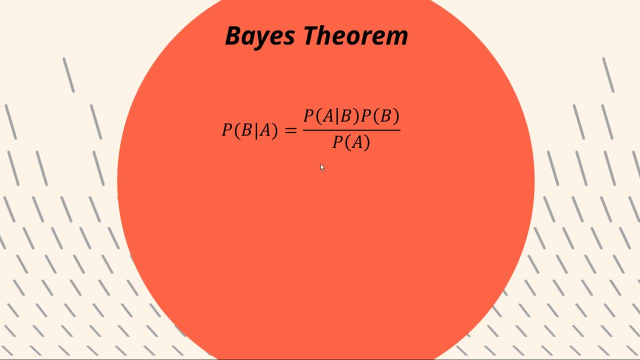 example they'll always give, which I'm surprised I haven't done in this particular video, But you might see that elsewhere if you have a look at Bayes' theorem applied to health stats. So let's have a look at the second example. Now, instead of A and B, I'm going to use Theta and 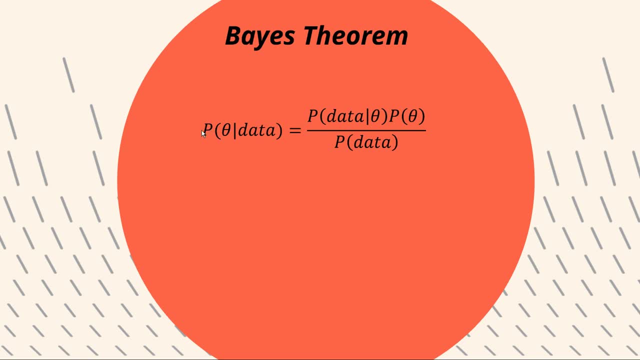 Data here. So it's exactly the same thing. but I'm saying here, the probability distribution of our parameter given our sample, or the data from our sample, is some function of the probability of getting our particular sample given a particular value of Theta And then times the probability of 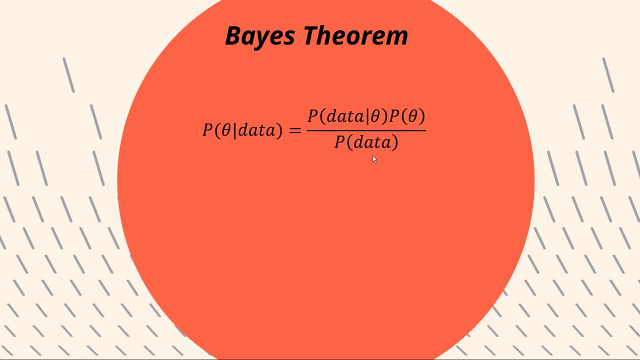 Theta divided by the probability of getting our sample. Now we need a little bit of lingo here when we deal with Bayes' theorem. So this particular part of the formula is called the prior. So this is essentially our prior intuitions about the parameter value. It has nothing to do with our 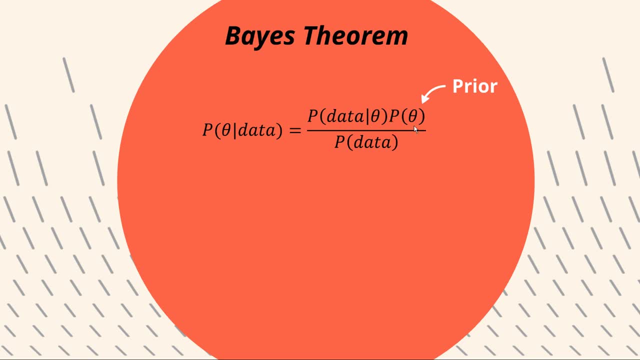 sample right, So we can actually construct this without having conducted our sample in the first place. Now the next piece of terminology we need to know is that this is called the posterior. If that's the prior distribution, this is the posterior distribution, which is the distribution. 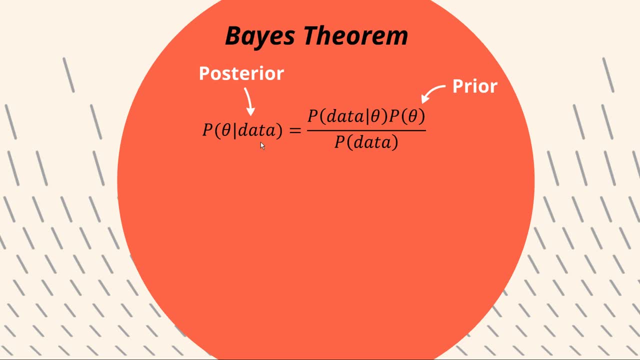 of Theta taking into account our sample. So once we've actually fed our sample into our little algorithm here, we can update our prior and turn it into something called a posterior probability, or in total you can call it a posterior distribution. Now this little thing in here is called a. 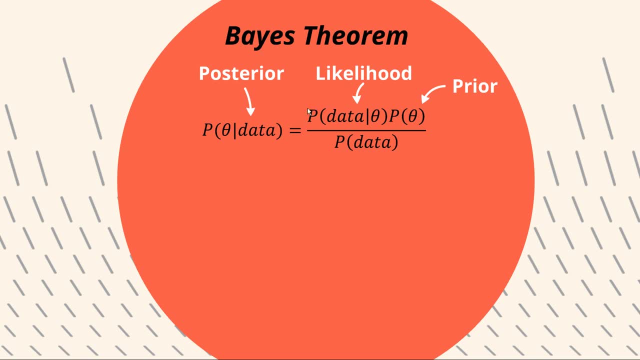 likelihood, and we've dealt with this in previous videos of this series of speaking. We're here to this series. This is just a distribution of possible sample outcomes for every given possible value of theta. And finally, on the denominator: here this is some kind of normalizing constant, The reason being, when you multiply your 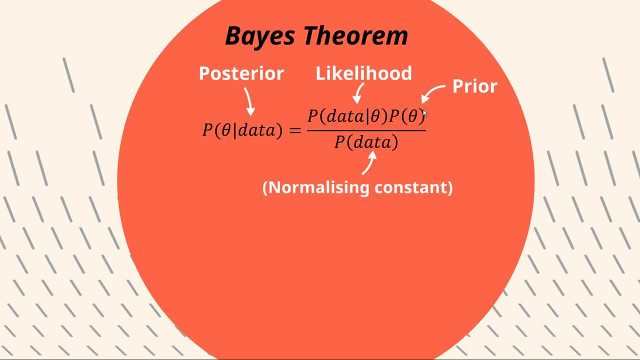 likelihood by your prior distribution, it doesn't necessarily follow that the resulting distribution will sum to 1.. So this normalizing constant just makes sure that our posterior distribution will sum to 1, which is important because, don't forget, this is a probability distribution. So without this, 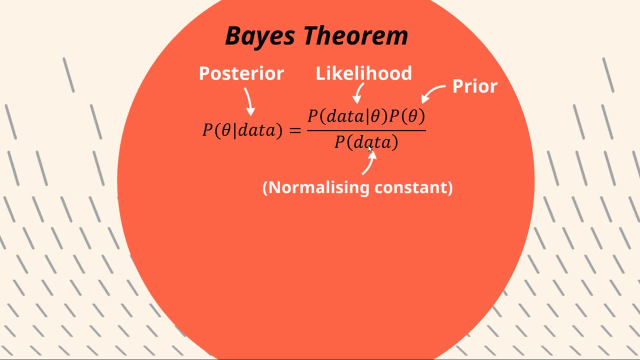 normalizing constant. it's technically not a probability distribution. Now, the cool thing about the normalizing constant, which is the thing on the denominator here, is that it's got nothing to do with theta, So in that sense we can kind of ignore it and say that the posterior distribution 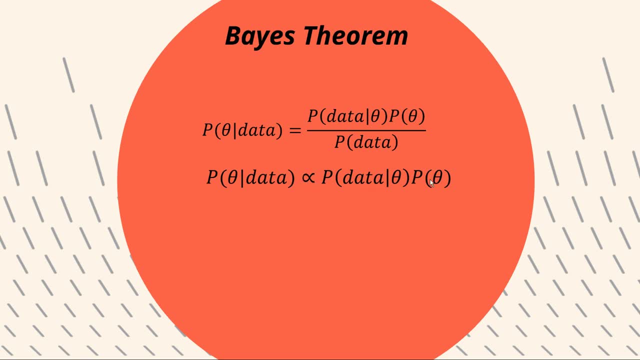 is proportional to the likelihood times, the prior distribution. So much like in the previous videos of the series, we don't really care about the scale of our probability distribution here, Given that our normalizing constant was just a constant. all it was really doing was multiplying everything by a particular 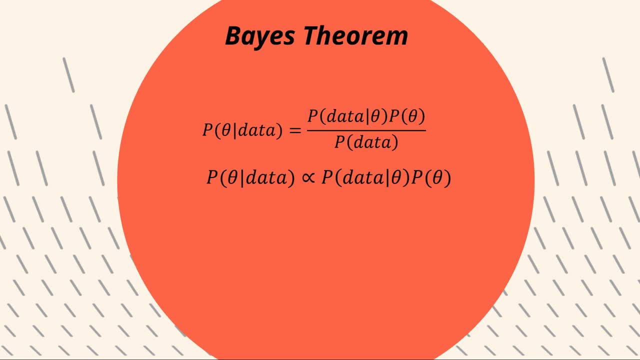 value. So if we eradicate that, we'll still find the same solutions to all of our problems. right When we try to find the same solutions to all of our problems, right When we try to find the same solutions to all of our problems, right When we try to. 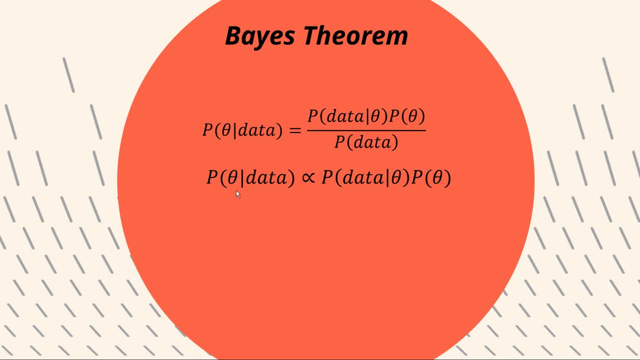 find the maximum value of theta, the maximizing value of theta. we can ignore all the constants in these equations, So that's why we get this nice, simple and very powerful relationship between this thing called a posterior distribution- our likelihood- and then a prior distribution. 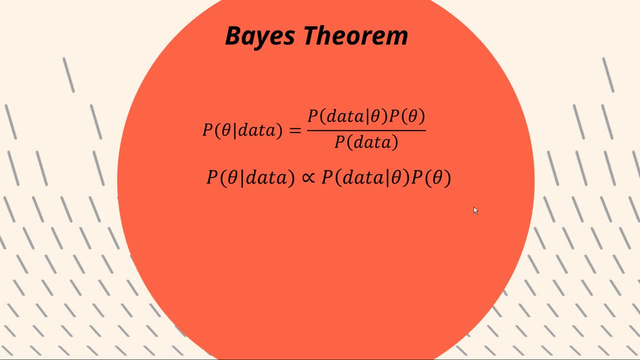 So just to summarize all that, Bayes Theorem is simply updating our prior intuitions about the parameter with information we gather from our sample, And then it becomes a question of how much do we weight our prior intuitions versus how much do we weight the information we get from our sample. 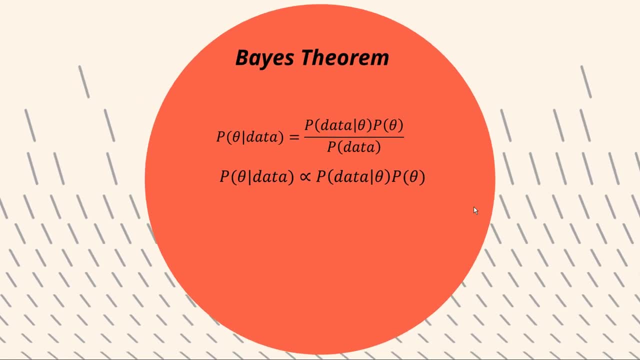 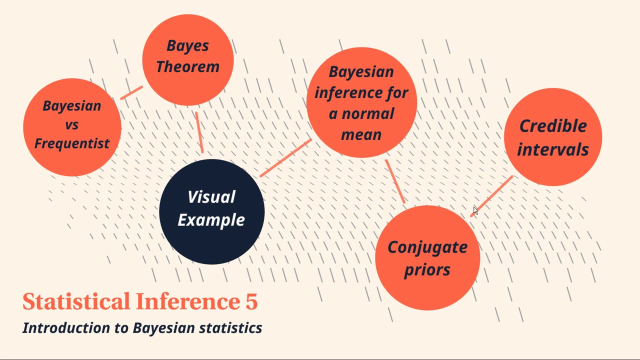 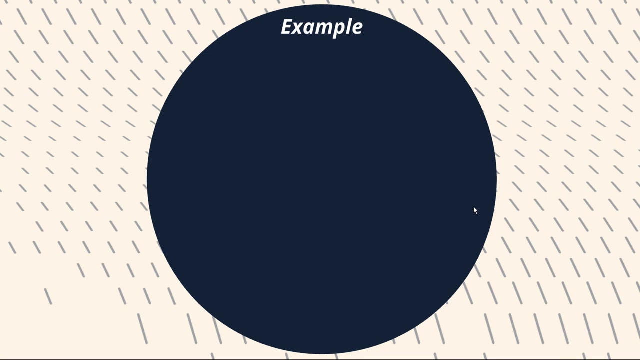 And that's what the rest of this video is going to be dealing with. All right, So that's enough theory for the moment. Let's tuck in to this visual example And, as I promised at the outset, this is going to lock in a real good sense of intuition. 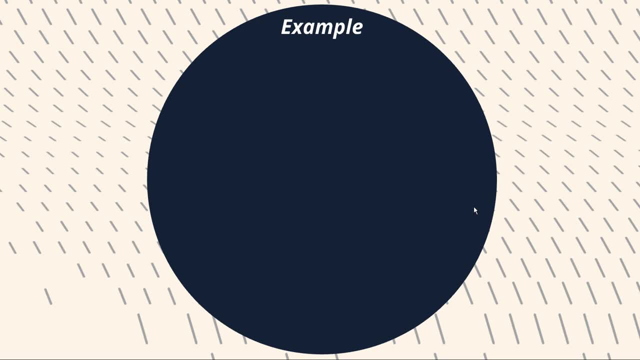 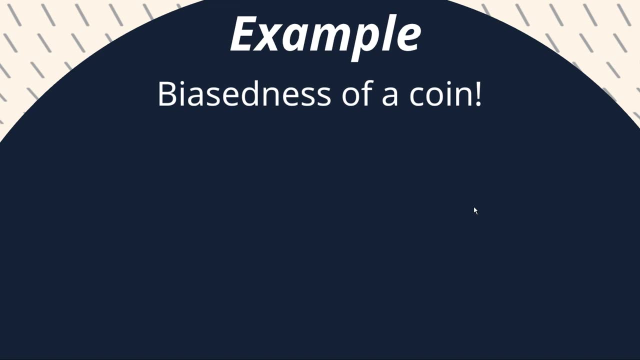 for you if you haven't got it already. So here's my example. It's a very simple example to do with the biasedness of an ordinary coin. Sorry, I couldn't be more adventurous with this, but I just think. visually it just makes. 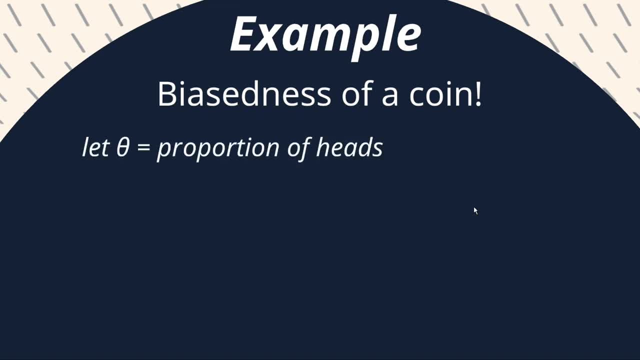 the most sense. So you'll have to forgive my lack of originality here. So let theta equal the proportion of heads that you get from a set of tosses of a coin. Now, if you're trying to assess the biasedness of a single coin, you might start out by thinking: 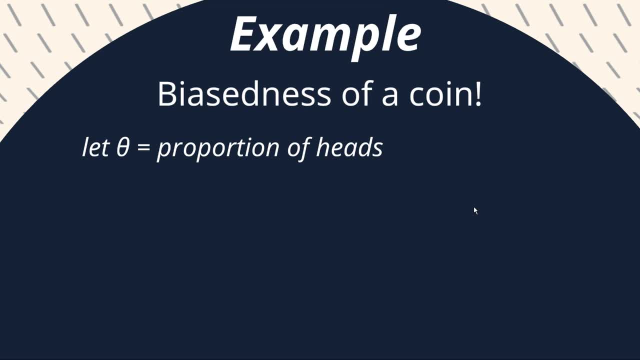 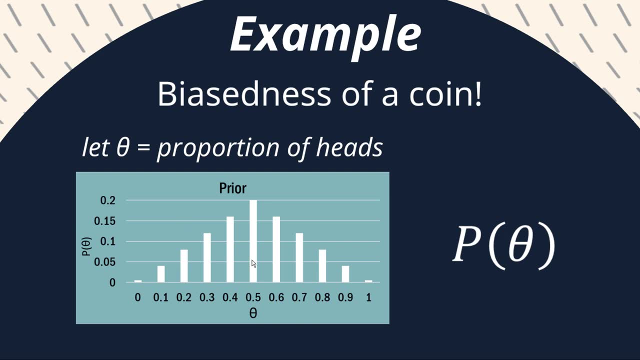 that that coin is unbiased. But what does that actually really look like? This is an example of a prior distribution where we have some inclination that this coin is going to be unbiased, such that 0.5, so 50% of the flips will turn out to be heads. 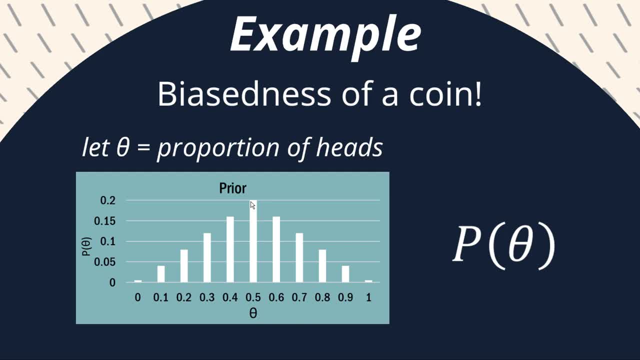 But let's just think about this. Let's just say that we're not completely convinced that this coin is going to be unbiased, So we're going to have a distribution about our prior intuitions. So what happens now is that we take a sample. 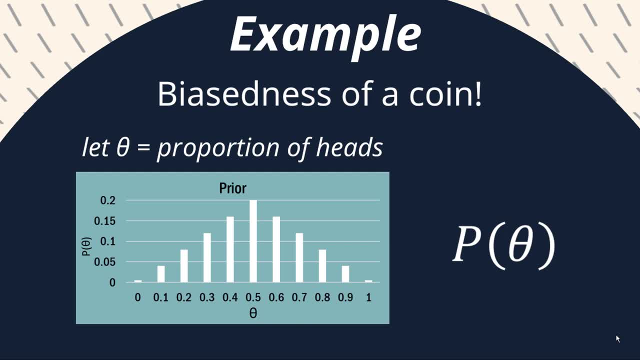 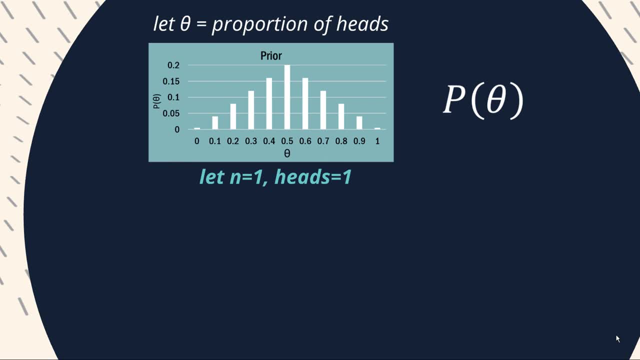 So let's take the simplest example you possibly could, which is just flipping one coin. Now, let's say, we've flipped one coin and it's turned out that it's heads. Now, how will this single piece of information we've gathered affect our prior predictions? 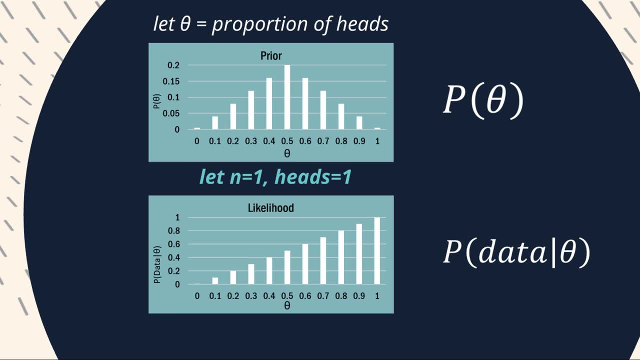 Well, we can construct now a likelihood distribution for each respective value of theta. So what this means is that, say, if theta was 1, so if this coin was so biased that 100% of flips turned out to be heads, then of course the probability of getting a head 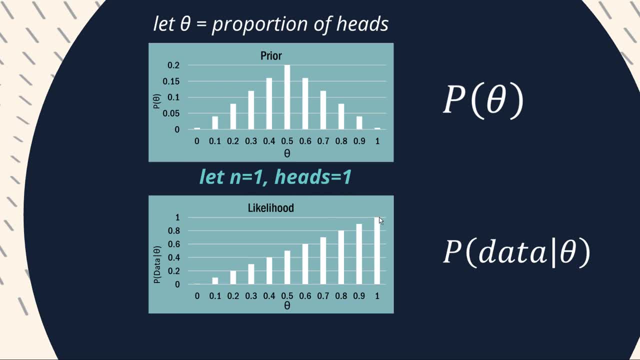 out of one flip would be 100%, But if the coin was only so biased that 90% of flips turned out to be heads, then of course the probability of getting the data that we did was 90%, so 0.9.. 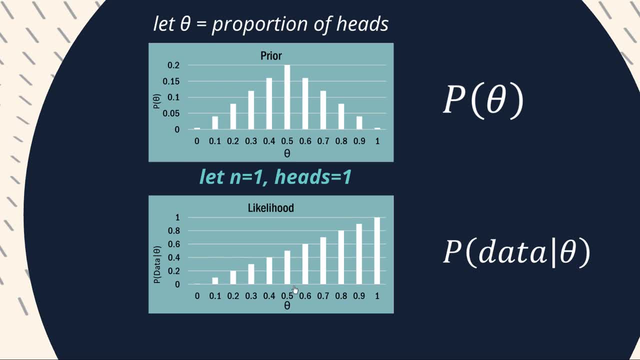 So you can see this is going to be a 1 to 1 relationship, right? So in the event that the coin was unbiased, you've got a 50% chance of getting that data that we just got. So in this piecemeal way. 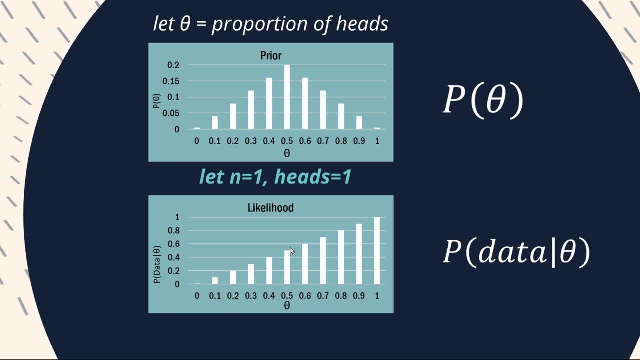 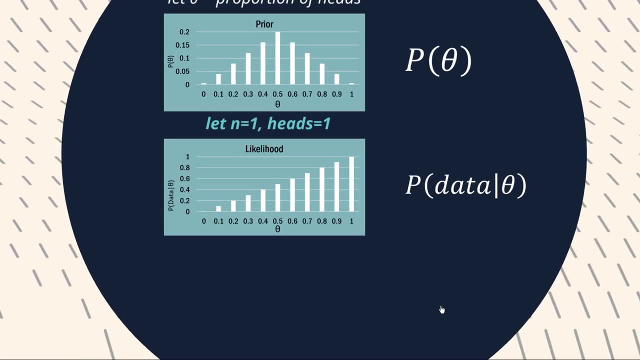 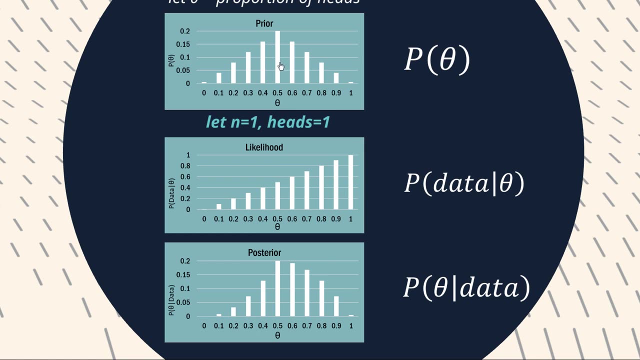 values of theta can be assessed for their likelihood of generating the sample that we got. Now the posterior distribution is just some manner of product between these two distributions. So, even though our prior indicated a very symmetrical distribution, once we incorporate the likelihood, which is 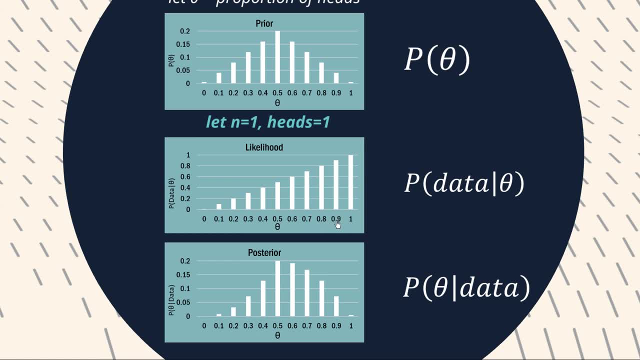 weighted more heavily up to the higher values of theta. you can see that we're going to get a bit of a skewed posterior distribution And essentially what's happening is that we're multiplying each pairing of these two bars together, So 0.5, we're multiplying the height of this bar up here for the 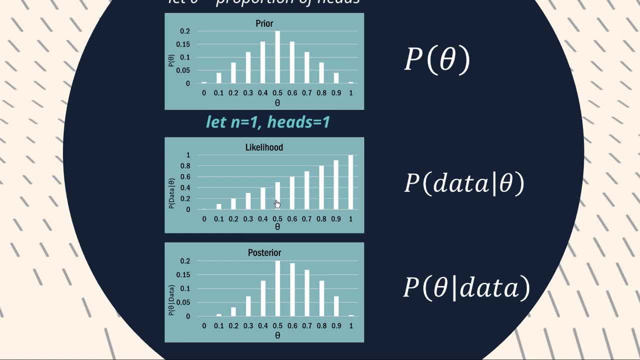 probability in the prior to this likelihood, and the same will happen for 0.6 and 0.7 and 0.8, etc. But the posterior due to being a product of prior and likelihood becomes skewed. Now I mentioned a bit earlier that it's some measure of a product, The reason why. 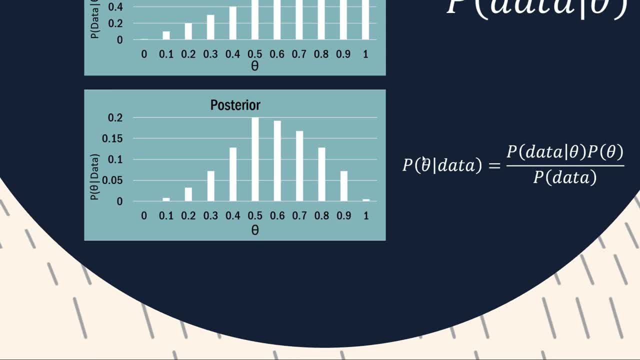 it's not a pure product- is, again, because of this aggregation, constant. So we're essentially taking each of those individual probabilities from the likelihood and multiplying it by the prior, and then we divide by this period with 0.5.. So if you want to check my calculations and you divide everything. 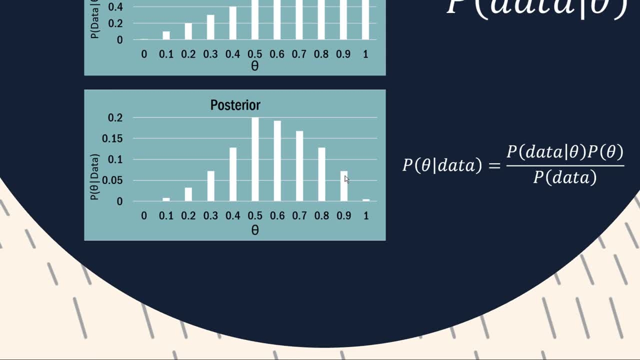 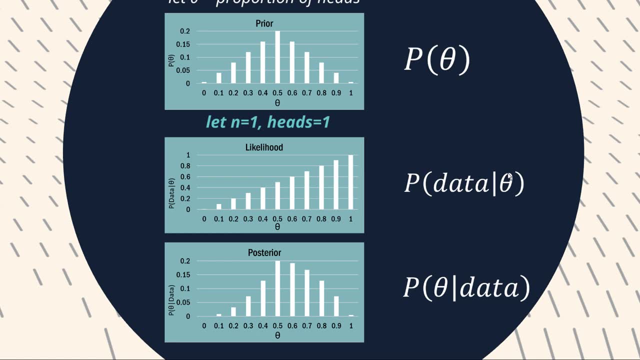 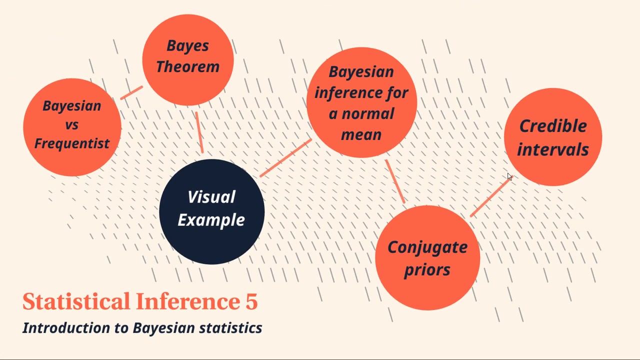 by 0.5, you'll hopefully sort of get the height of these bars Looking at pretty similar. But hopefully that's kind of given you a nice little picture of how Bayesian statistics incorporates prior predictions of our parameter value with a particular sample. that we've got Alright, so we're going to look at now Bayesian inference. for a normal 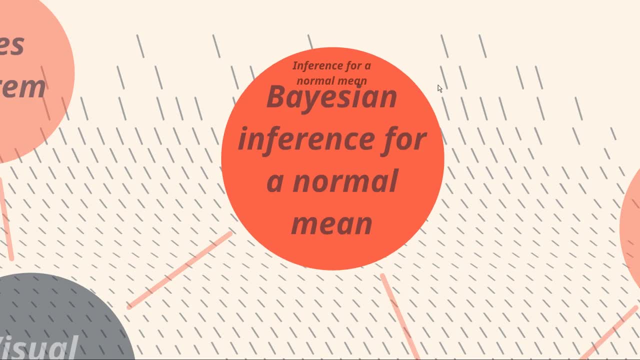 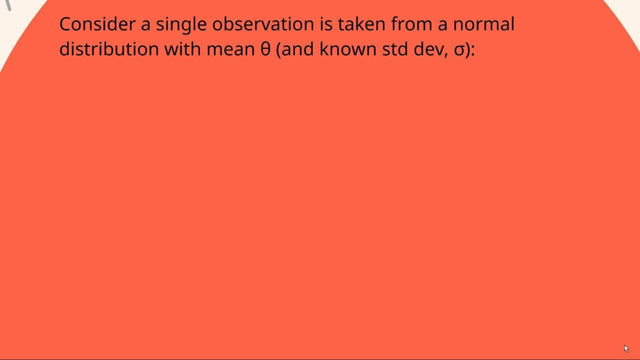 mean. So it's going to be a little bit more in-depth. So let's consider a single observation taken from a normal distribution with mean theta and known standard deviation sigma. Now I've simplified it by allowing the standard deviation to be known, So there's only one. 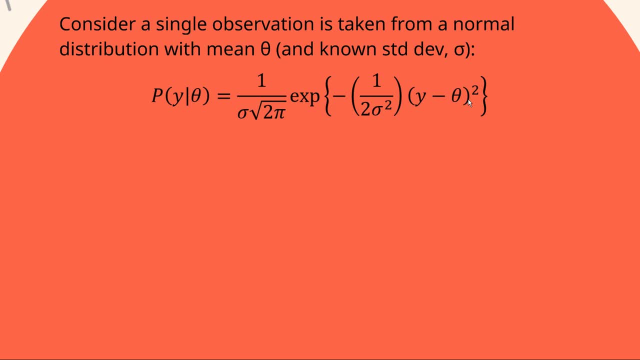 parameter of interest here, which is theta. Bayesian statistics can obviously deal with a situation where we have a normal distribution of theta and a normal distribution of sigma. So let's consider a single observation taken from a normal distribution with mean theta, And so I've simplified it by just allowing theta to be our parameter. Sigma is therefore: 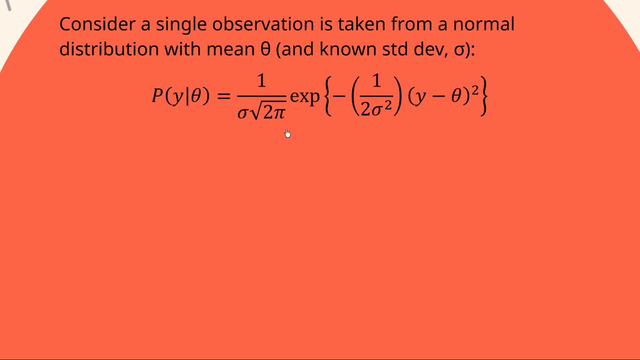 fixed as our variance or our standard deviation. Now, this is a likelihood. You might have seen it before if you've dealt with the PDF- the probability density function that emanates from a normal distribution. So, remembering our Bayesian relationship, we're going to 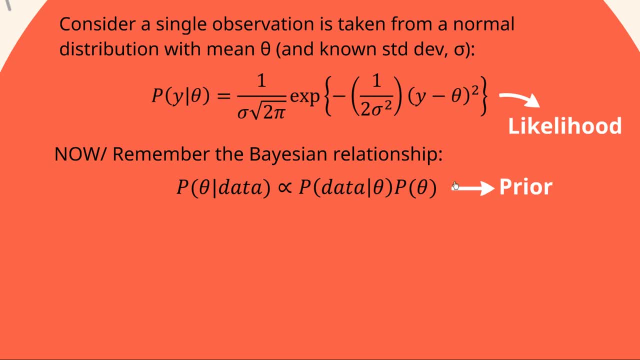 have a relationship where we've got the prior times, this likelihood equaling our posterior while being proportional to our posterior. We now have to consider what kind of distribution our prior is going to be. We have complete autonomy over that. We can create whatever type of distribution we want for our prior, But keep in mind that it has to eventually. 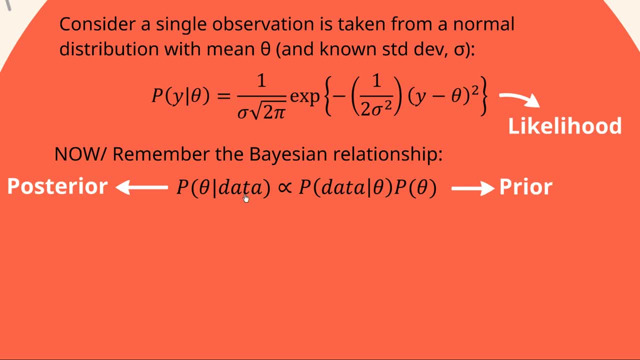 multiply with our likelihood to get our posterior. So here's just that expression, again using y instead of data, which is the same thing. I'm just using the letter y here to represent our particular sampled value. Let's consider a prior of the following form: So here we have again. it's in the exponential function. 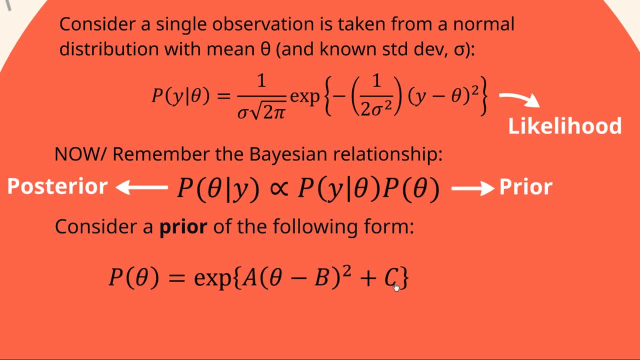 a times theta minus b, all squared plus c, Now that c is going to come out in the water. Now, if we take a ratio of c to the power of c to the power of c plus c minus c, We're assuming that c is going to be equal to c to the power of c. So what I'm going to do? 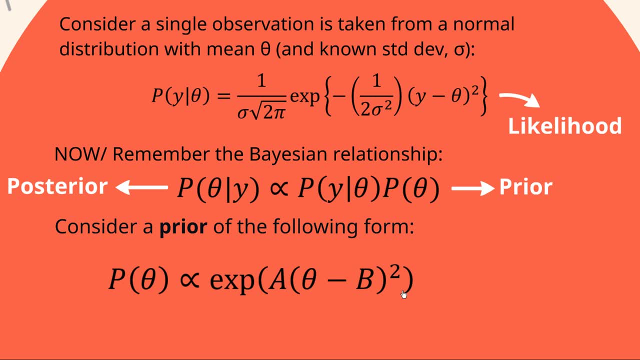 is, I'm going to take a ratio of c to the power of c plus c, and I'm going to take a ratio of c to the power of c. So in this case, c is the potential. We're going to multiply that. What we're saying is that we have gets to a factor of c to the power of c, but it's 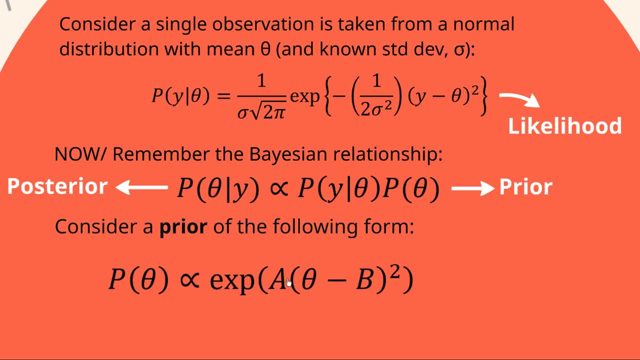 posterior distribution And before we do multiply it through, let's just re-parameterize this prior. So instead of having a and b, let's have tau and mu, two Greek letters, And the reason why I would have re-parameterized it to look a bit. 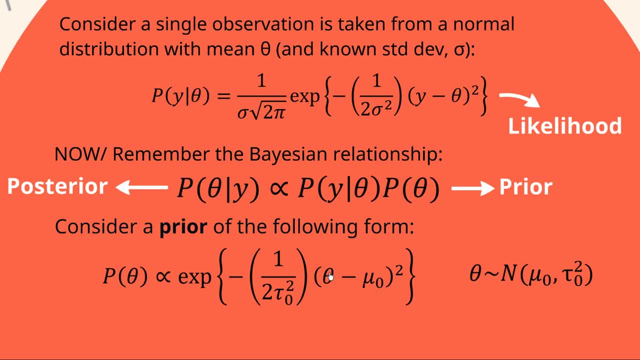 like this, as opposed to a simpler a times theta minus b, is that this is now in a form which represents a normal distribution itself. So here is a prior distribution which is normally distributed with a mean of mu and a variance of tau squared. Now I've put subscripts 0 here, because what we're 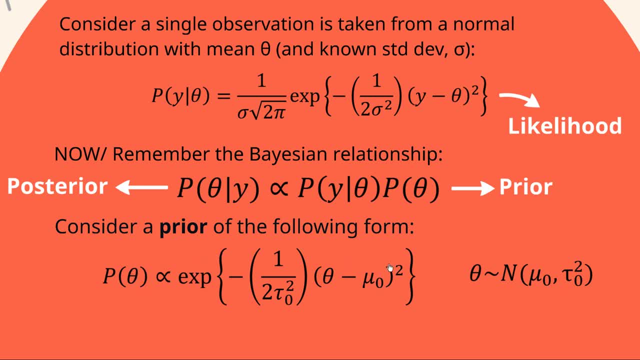 going to find is that when we multiply this prior distribution with our likelihood, we're going to get a posterior that looks very similar And that's indeed very handy. So let's see if we can get a posterior that looks very similar And that's indeed very handy. So let's. 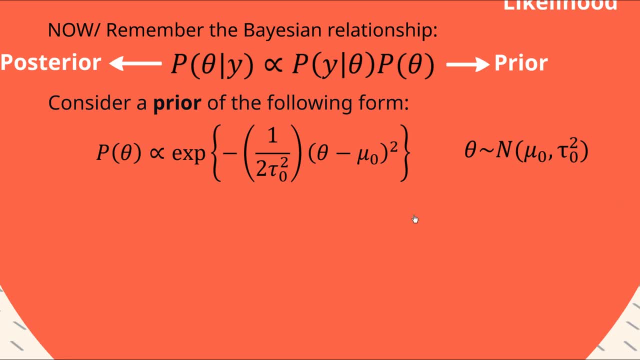 see how that plays out. Now, before we reveal what the posterior is going to look like, keep in mind that we're going to need a sample right, Because you need to multiply the prior by a likelihood. And what's a likelihood? Well, it's a likelihood of a particular 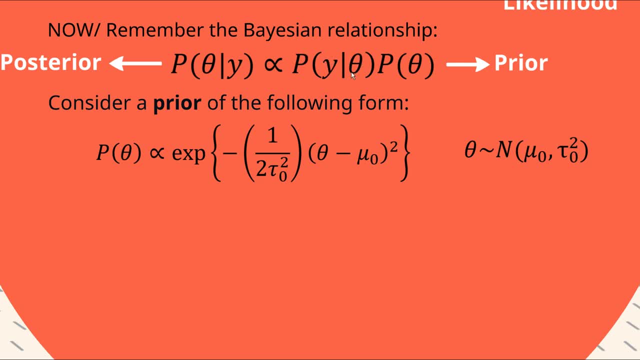 sample, given certain values of your parameter. So we need that sample. So for the moment, let's just presume the simplest sample possible, where our I have one value or one observation, which is y. So the posterior, given that it's the product. 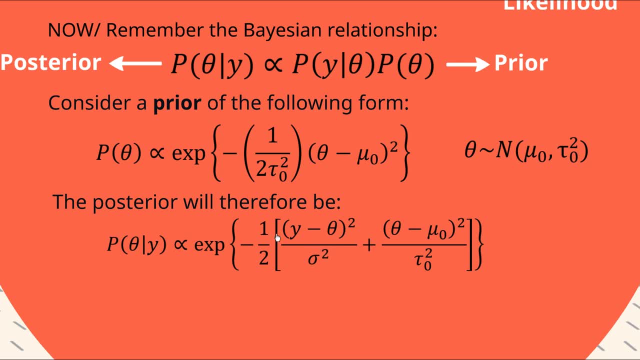 of this prior and the likelihood that we saw before. it's pretty simple, because we have two expressions within an exponential function that are getting multiplied together, so the indices just get added together. So we've got this first bit here from the likelihood and this bit over. 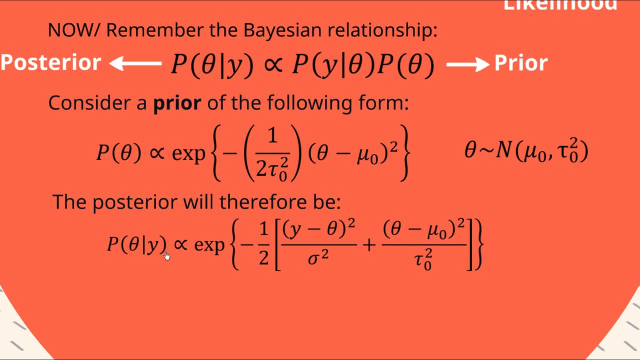 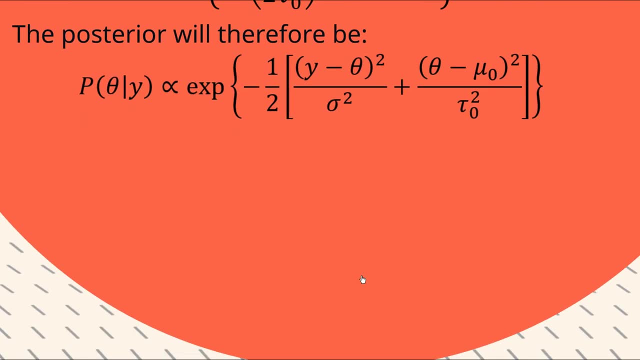 here comes straight from the prior, So our posterior will be proportional to this particular expression here. Now you can see I've got mu naught and tau naught here. What I want to do is I kind of want to try to express this in a simplified form, and I'll do that in this next. 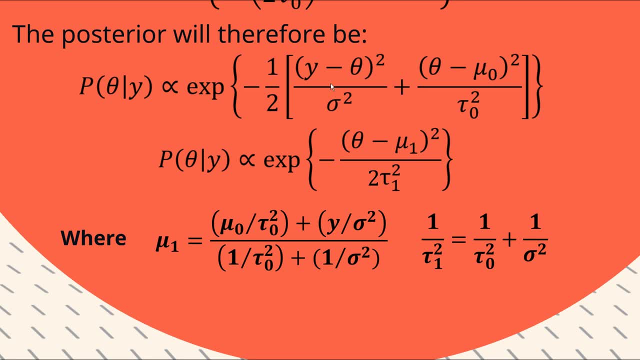 section here where instead of mu, naughts and tau, naughts and y's and sigmas, I'm changing it to mu1 and tau1.. And there's quite a bit of algebra that is required to get from this first one to this. 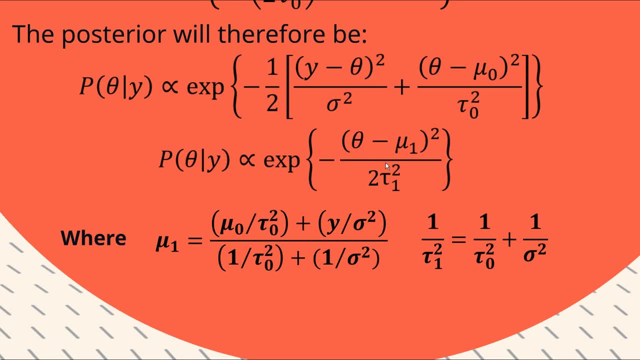 second one. But to spare you the agony of that, I've just done it behind the scenes. But believe you me, the values for mu1 and tau1 that eventuate are given by these two expressions here. So this is showing you the relationship between our new mu1 and tau1 versus the old mu naught and tau naught. 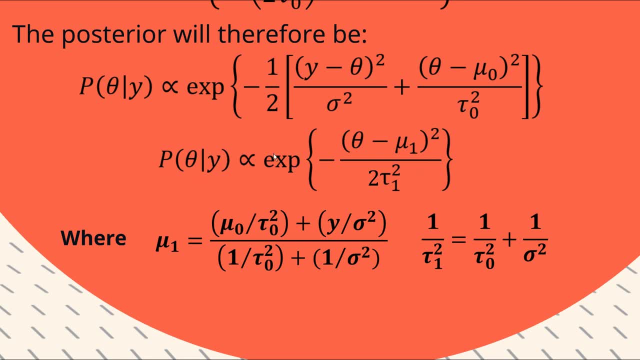 So, in other words, our posterior here is also going to be a normal distribution, because this is the form of a normal distribution, but it will have a mean of mu1 and a variance of tau1 squared where those two values are given by these two expressions. So let's first have a look at mu1.. 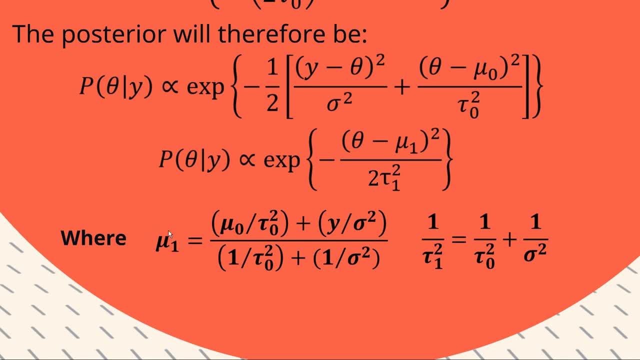 So, don't forget, this is the new mean or the posterior's mean, given a prior's mean, and also the prior's standard deviation. So this is the new mean or the posterior's mean, given a prior's mean, and also the prior's standard deviation. 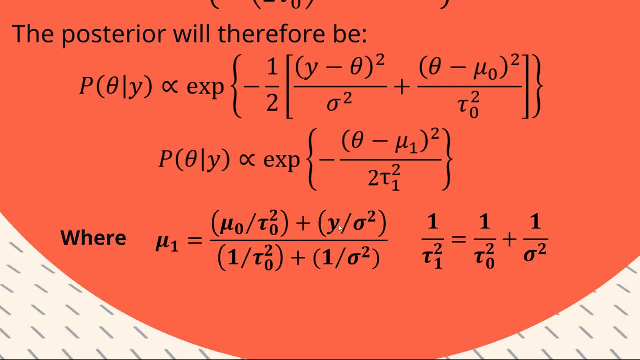 So this particular formula holds here for where we have a sample of size 1, and that's why I've called it mu1 and tau1.. So what's happening here is that our mean of our posterior distribution is some kind of weighted average of the mean from the prior. 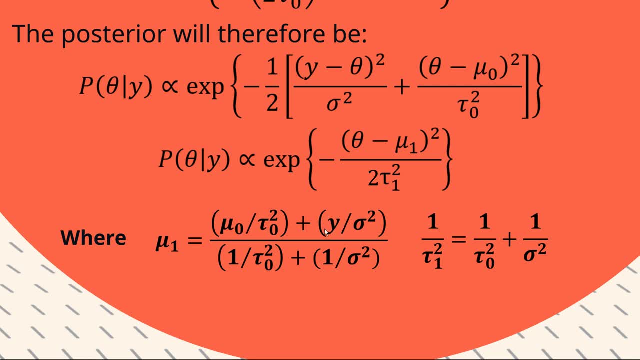 distribution and our single data point, y. You can see that y is kind of scaled by its variance and the prior'sем an inch, the mean of the самиモ" isscaled by its variance and the prior's mean and the variance squared. 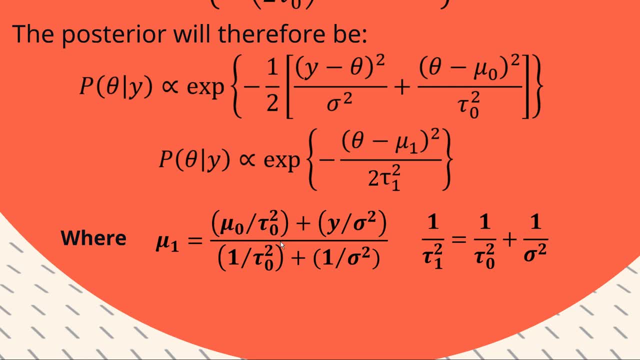 and the prior's mean and the variance squared is a Townsend point, point y and synecdoches. what is that? mean is scaled by its variance And furthermore, you can see that 1 on tau, 1 squared. so this is the precision. When you have 1 on a variance, we can call that the precision. So this is. 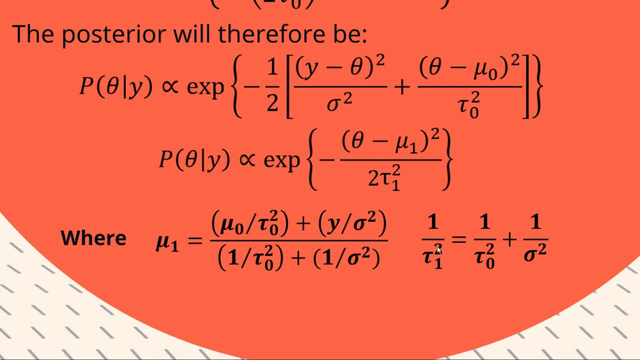 the precision of our posterior distribution. It's again some kind of average of the prior's precision and the precision of our sample, which just happens to be of size 1 for the moment. So you can see what's going to happen if our variance of our prior distribution 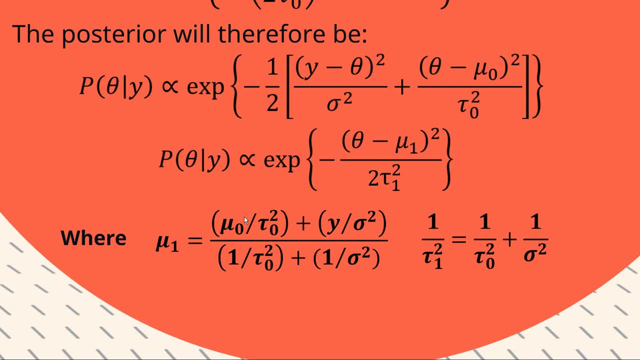 is quite high, then it's going to tilt this weighted average in favor of our sample's value. But, on the contrary, if the variance of our prior distribution is quite low, it's going to take a while for our posterior to budge away from that mu naught value and the 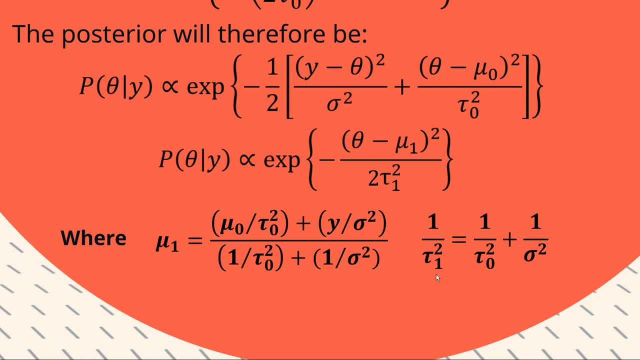 same could be said for the precision over here. So I'll repeat that it's a 1.2 squared. So the same could be said for the precision over here. So I'll repeat that It's a weighted average of our prior distribution and the sample that we got. 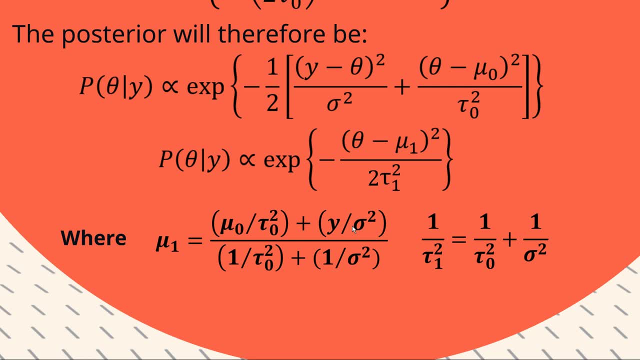 Now we can generalize this to a scenario where there's more than one observation in the sample, and let's just say there are now n observations in the sample. so these formula will change. It's the same posterior distribution up here, but if, instead of using mu1 we use mu n, which is now the mean for a posterior 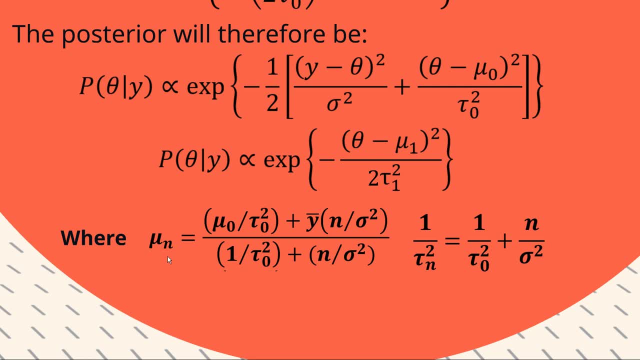 distribution after generating a sample of size n. everything's the same, except we now have these factors of n in here with the samples mean. And similarly, on the precision side, instead of one on Sigma squared we now have n on Sigma squared. So not only do we have an effect of the respective variances here in 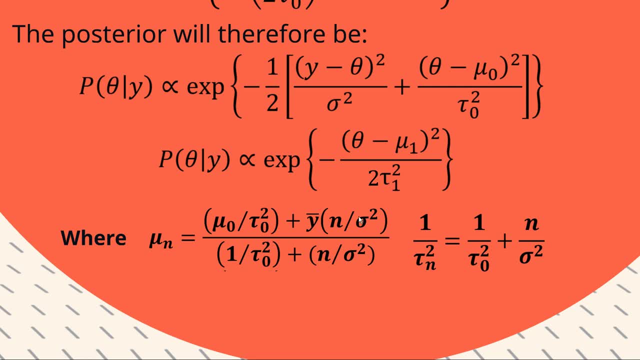 terms of, in terms of how this average is being weighted. but we also have the factor of size, this factor of n. So if our sample size increases, our posteriors mean will start gravitating to that samples average. The weighting becomes more heavily tilted to the side of the sample, away from the prior. 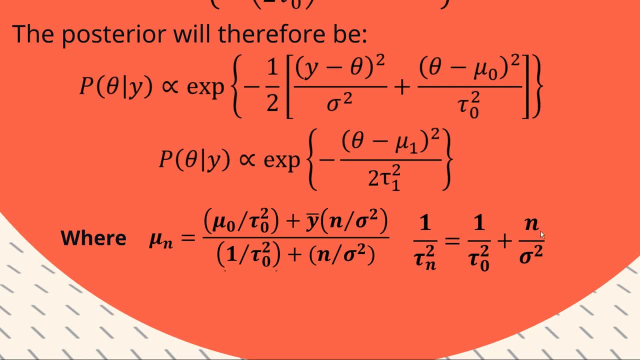 distribution. Similarly, with our precision, if n becomes a lot larger, the precision is going to be weighted more heavily in favor of Sigma squared, which is the known variance from our sampling, as opposed to our priors variance. Now I should have maybe updated this formula up here to write mu n and tau n up. 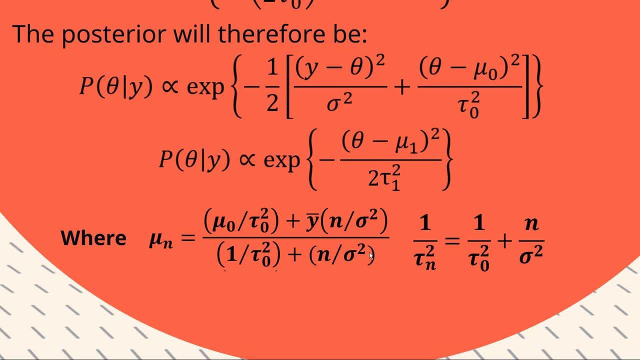 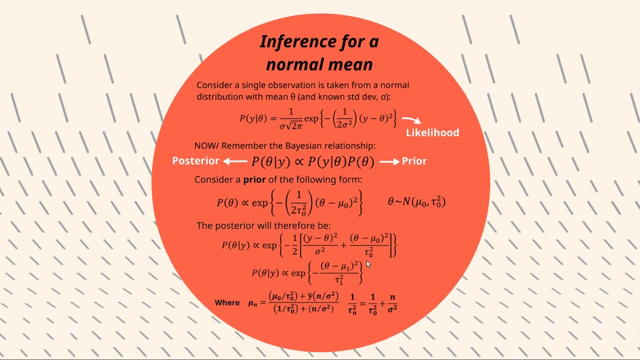 there, but you can try to visualize that yourselves. But hopefully that's given you a nice little window into how a posteriors mean and precision or mean and variance, is just a weighted average of the prior distribution and the likelihood of generating our specific sample. All right, let's move on. So let's. 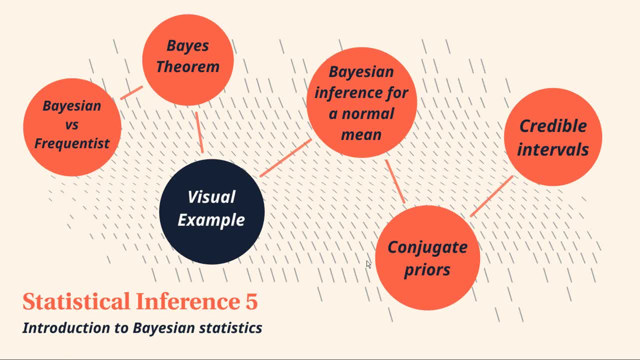 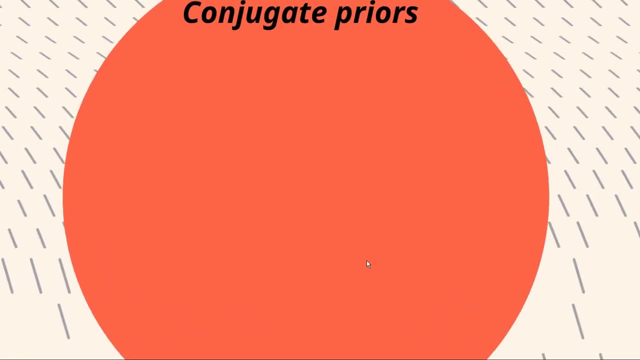 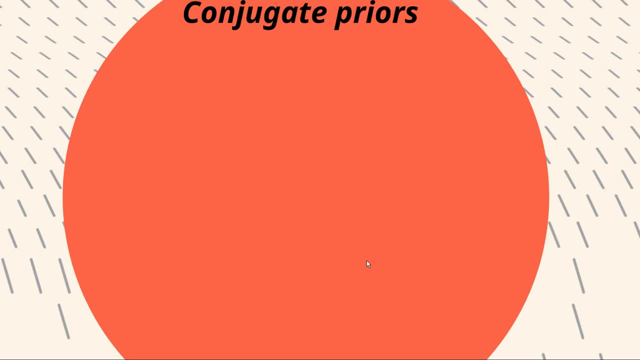 Remember the way we were comparing mu 1 to mu n and tau 1 to tau n and considering how it's like a weighted average of all that stuff. Well, that only could happen because we were dealing with the same distributions on both ends, for prior and posterior, And when that happens we say that the prior is a. 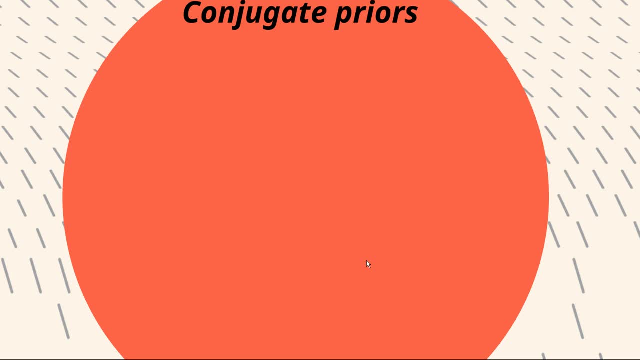 conjugate prior because it creates in the posterior the same distribution. Let's have a look at the Bayesian equation again. I'm not going to go over that for a third time, but we often choose convenient parametric forms for our priors such that the posterior remains manageable. 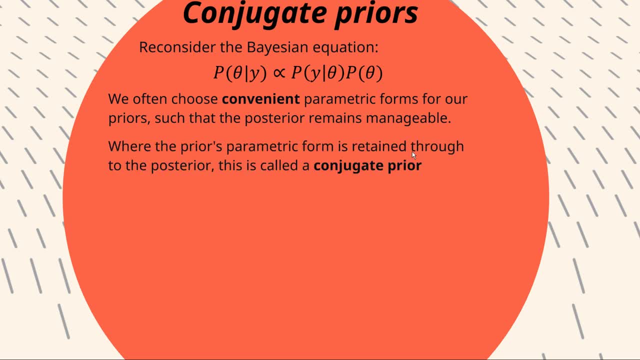 And, as I said before, where the priors parametric form is retained through to the posterior, this is called a conjugate prior. So don't be confused. this is not to do with the likelihood, but if a particular prior we choose eventuates in the same distribution. So if we choose a particular prior, we choose a particular. 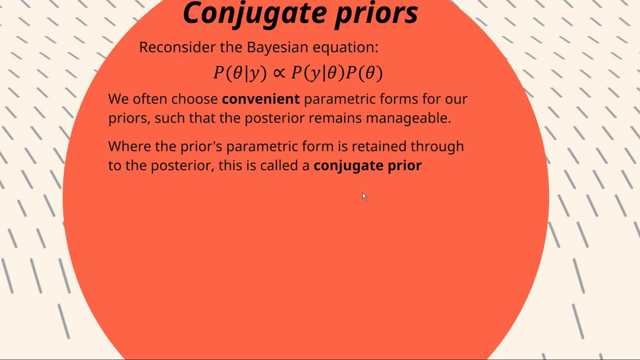 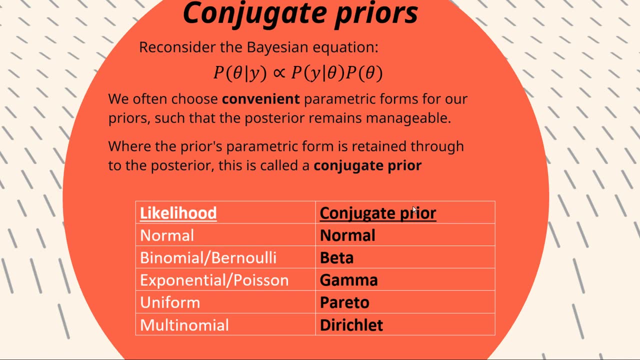 distribution. for our posterior we say that that prior is a conjugate prior. So what I've got here is just a list of likelihoods with the particular distributions that would be conjugate for the prior distribution. So when the likelihood is normal, choosing a prior that's a normal distribution will result. 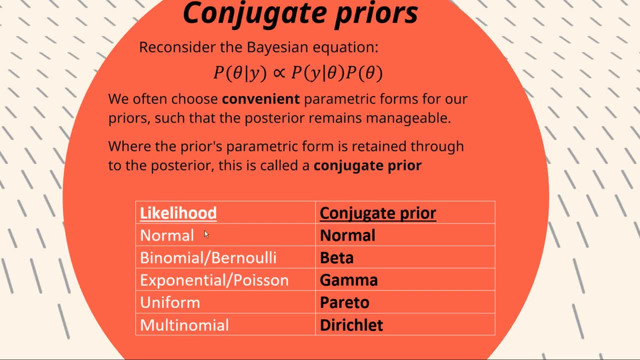 in a posterior normal distribution. Now this is actually called being a self conjugate, which doesn't often happen for other distributions. You can see that if our likelihood is expressed as a binomial or Bernoulli distribution, we need a beta prior distribution to result in a beta posterior distribution. So the 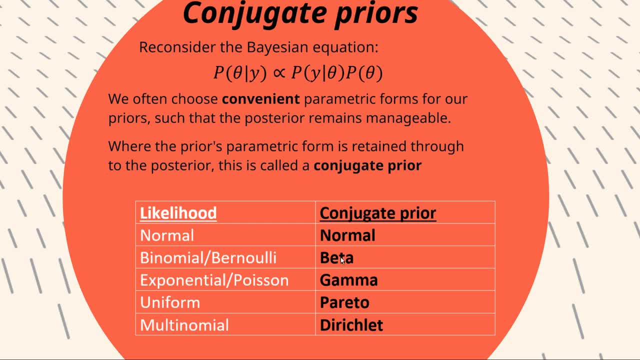 corresponding conjugate prior would be a beta distribution. So for exponential and Poisson it's gamma, and for uniform it's Pareto and multinomial it's something called the Dirac-Leigh, which I'm sure is a French statistician from a bygone era. 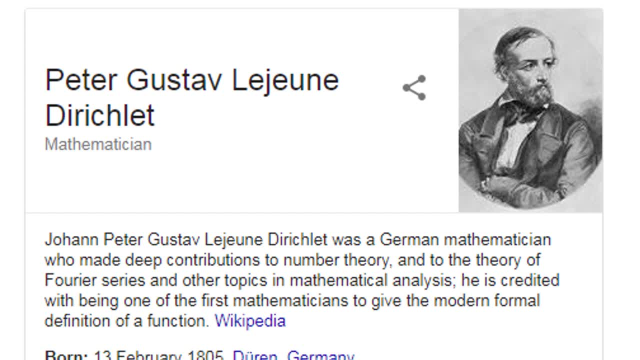 Okay, so it's Justin here just editing this video and interrupting momentarily to let you know that I was full of it when I said the guy was French. Turns out he's German, definitely from a bygone era. Do a little research, Justin, before doing the first run. 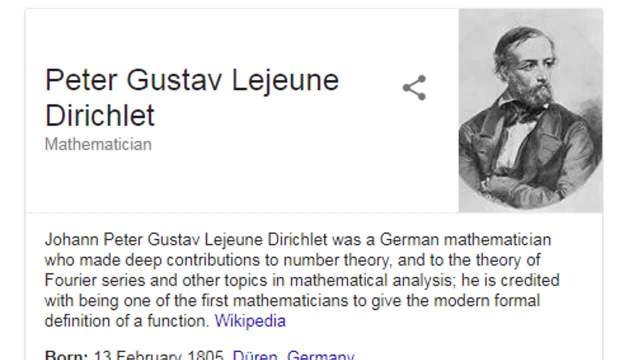 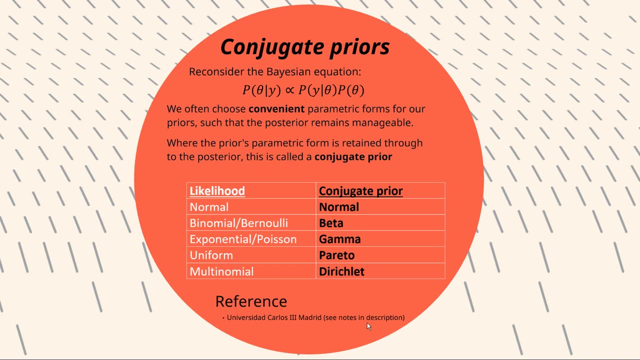 of the audio. That's my lesson And I also like how I pronounced it in a very French way, just to show how culturally aware I am. Anyway, Back to the show. If you're keen on diving a little deeper into conjugate priors, I'll leave in the notes of 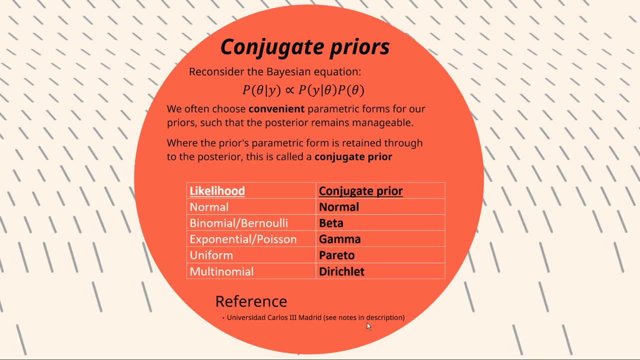 or in the description of the video a link to these lecture notes I found online from Carlos III University in Madrid. They're written in English, thankfully, but they were quite useful when I was trying to do a little research to figure out. you know what these combinations. 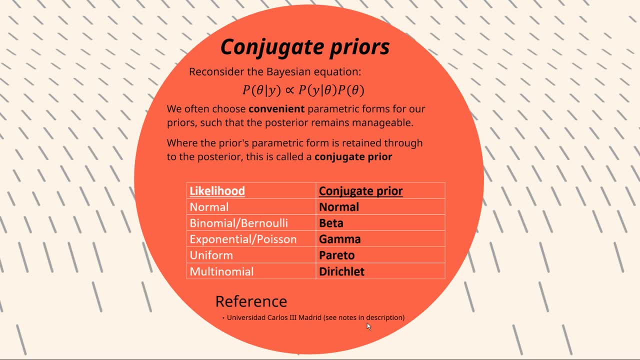 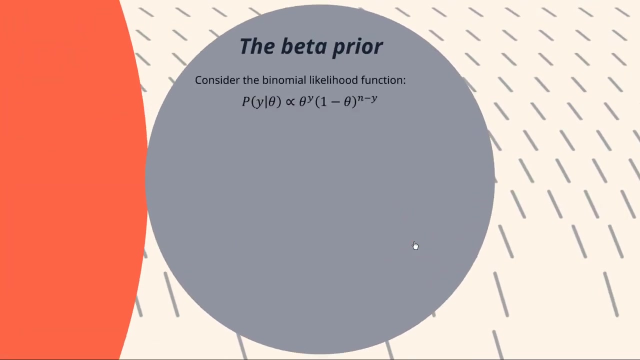 of likelihoods and conjugate priors were. But I'm not going to let you escape that easily. We're going to have a look at the combination of binomial likelihood and choosing a beta distribution for our prior to allow it to be conjugate. So let's do that now. Let's have a look at the beta prior. 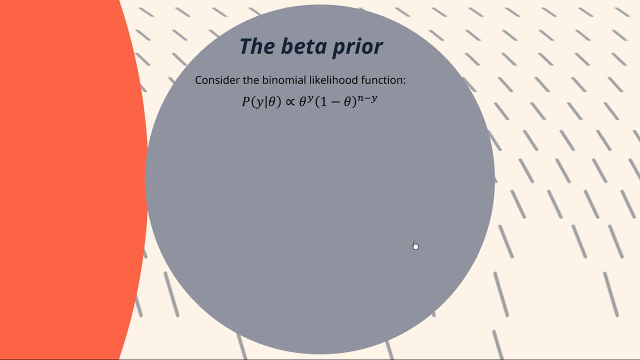 So let's consider a binomial likelihood function, which you would have seen in your studies prior to this, hopefully- Where you've got your parameter to the power of 1. And you've got your parameter to the power of 1. And you've got your parameter to the power of 1.. 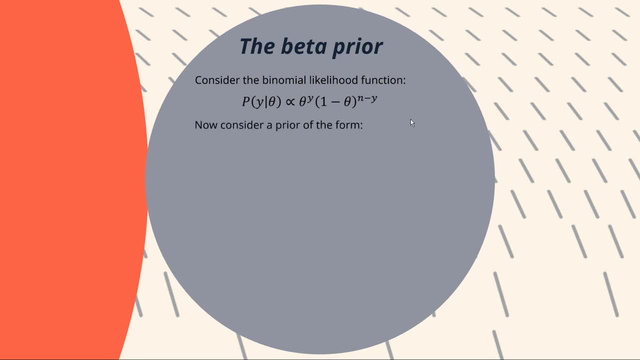 courageous is N minus Y and then 1 minus the parameter to N minus Y. So let's consider a prior of this form, which looks almost exactly the same, which is theta to the power of something times 1 minus theta to the power something else. 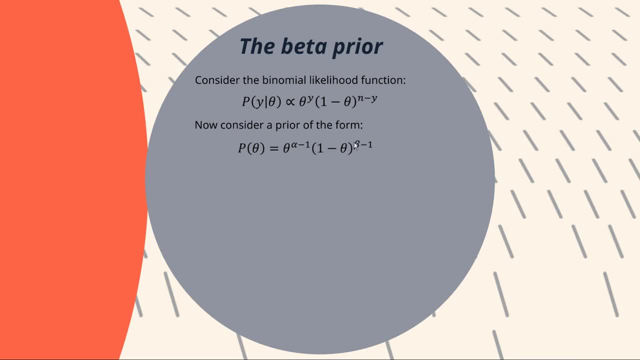 Now, the convenience of choosing something in this form is that, like with the normal distribution, when you multiply this with the likelihood you're actually going to get a very easy calculation. itself will be of the same form, But the only problem with this is that this: 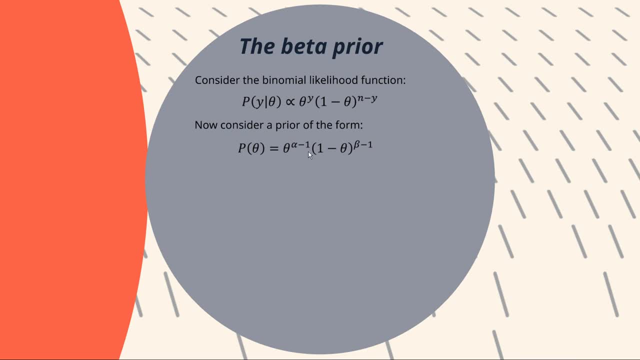 doesn't necessarily result in a probability distribution. What do I mean by that? Well, the total probability density across all combinations of alpha and beta will not sum to one, And that's a problem, because a prior distribution is a prior probability distribution. so while it's well and good to say that the 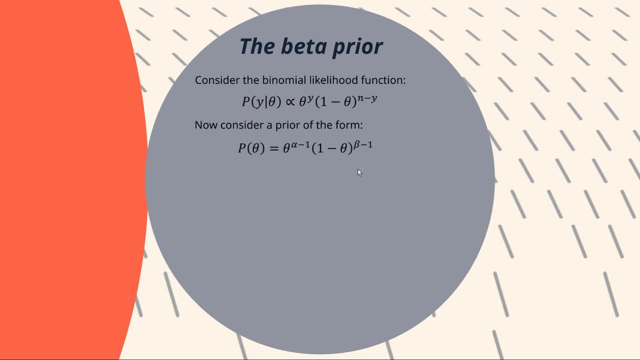 prior needs to be of this form? well, it still needs to be a legitimate probability distribution. So to do that, we divide by this thing called the beta function. So this itself is called the beta distribution, which could get a little bit confusing. So let's try to get our terminology correct from the outset. 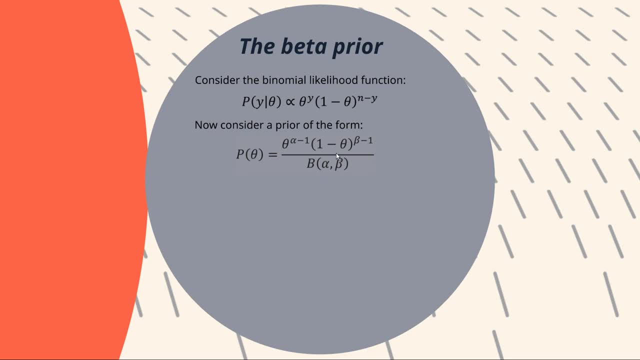 This is called a beta distribution, part of which is this beta. This is actually an important number. This is an important number because it beta function of alpha and beta. But again, this beta function just acts as some kind of normalizing constant. you can say: The parts of this prior distribution that deal. 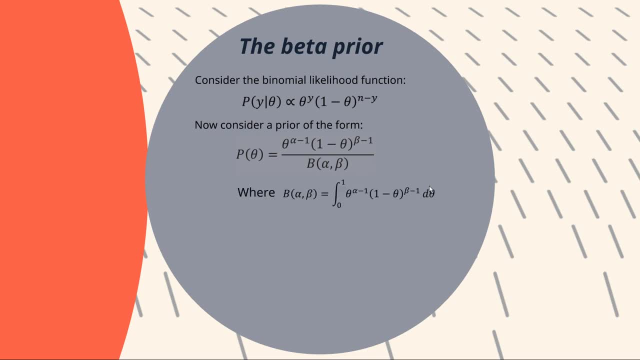 with theta are on the numerator. So for the nerds out there, this beta function is actually just an integral of what's on the top here between 0 and 1.. So essentially it divides by the area under the curve right. Remember your calculus from school, your geometrical? 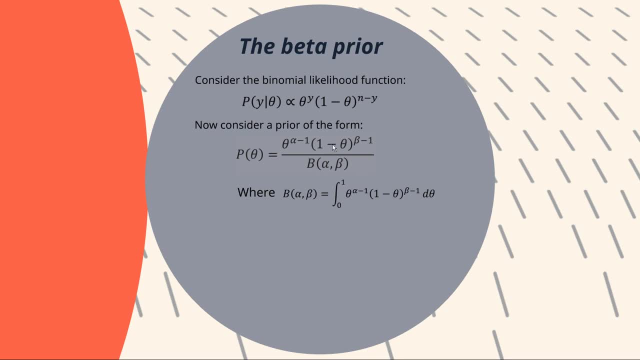 applications of calculus. By dividing by the area under the curve, we ensure that the resulting distribution will sum to 1.. So let's now actually write the posterior. It's the product of the likelihood function and this new beta distribution. Now, as you can see, I've actually ignored the beta function, because 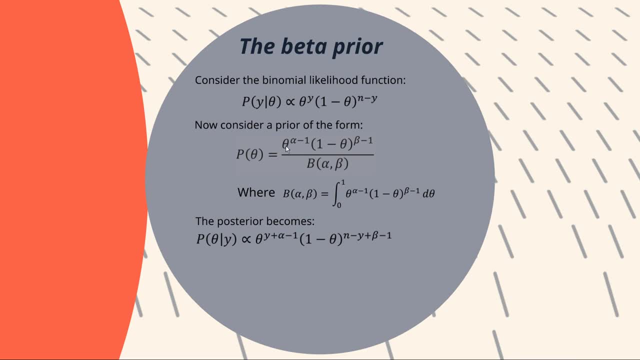 as I said before, it's essentially a constant. It's got nothing to do with theta. So our posterior is proportional to this theta, to the power of y plus alpha minus 1, and then y minus theta, to all this stuff here. So you can see our posterior is actually still. 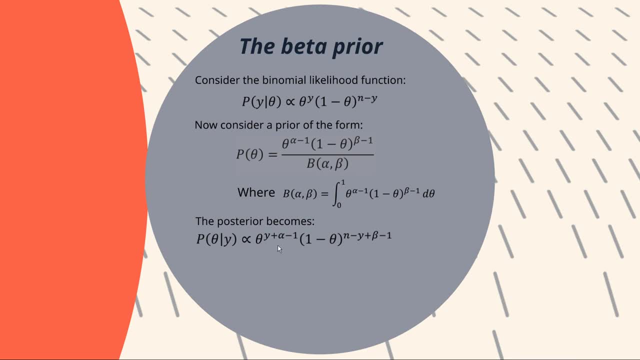 in the same form as our prior, which is very convenient. Subtitles by the Amaraorg community. Now, the reason why I've chosen this one to highlight is that you can see, hopefully, the relationship between the posterior here and our original likelihood function. The. 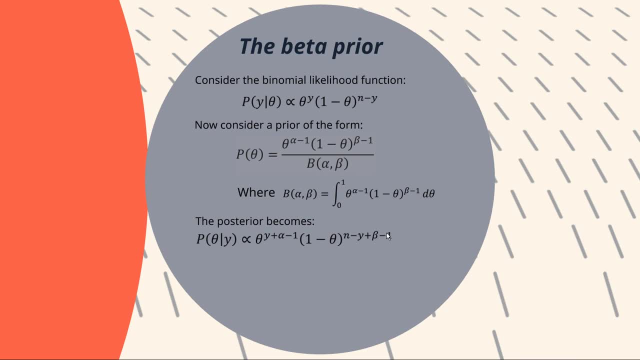 difference is only these alpha minus 1 and beta minus 1 characters. So if this likelihood function represents what's happening in our sample, our posterior represents a sort of combination of what's happening in our sample and what we've presumed from our prior distribution. 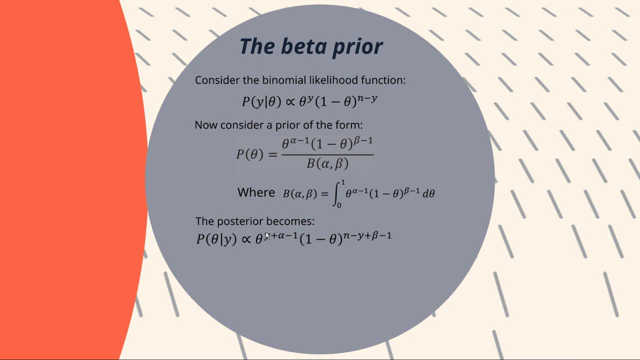 So we've got again two components- the y component or the n minus y component on this side, and we have this alpha and beta component which comes from our prior. So in other words, the prior distribution is essentially analogous to having alpha minus. 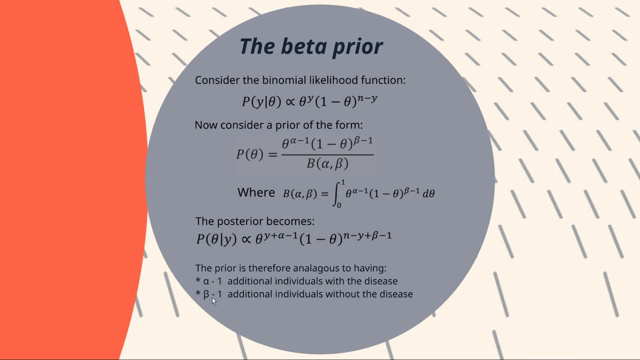 1 additional individuals with the disease and beta minus 1 additional individuals without the disease. Now I've assumed here that theta is the probability of disease. So I've assumed here that theta is the probability of developing some kind of disease here. but you could. 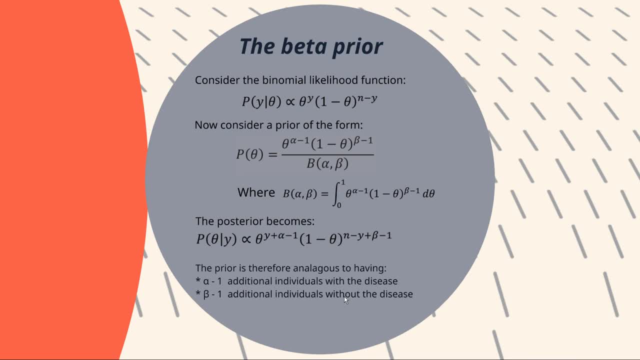 just put with the event and without the event, if you want to keep it general. So all you need to do is select a value of alpha and beta respectively, and you're essentially adding some individuals into your sample. Now, what's the effect of sample size if your 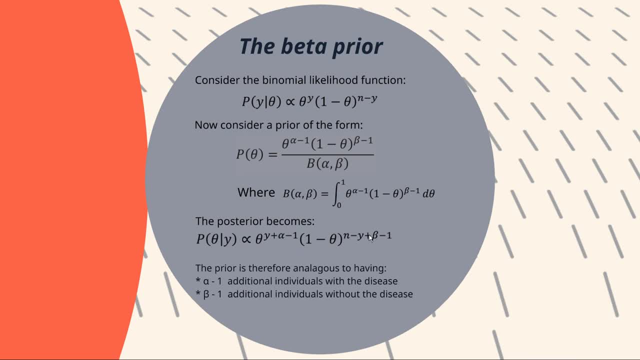 sample size increases for a given prior distribution. So say, alpha and beta is fixed, but your sample size is now increasing. quite clearly your posterior is going to lean more heavily towards whatever's happening in your sample. So again that nice sort of weighting happens. 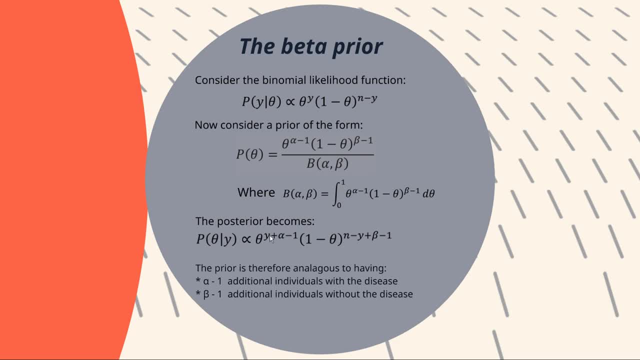 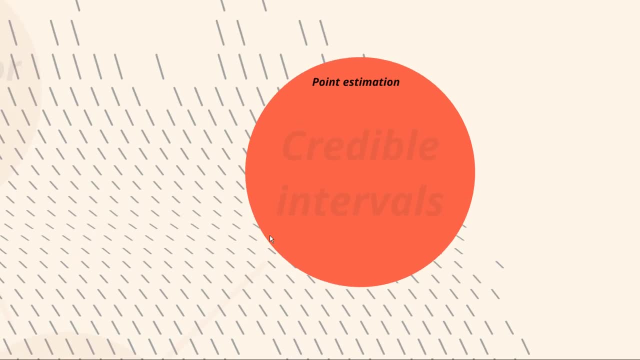 between sample and prior. All right, So the final little piece of the puzzle is looking at credible intervals, which is the Bayesian equivalent of confidence intervals. All right, So the final little piece of the puzzle is looking at credible intervals, which is the Bayesian equivalent of confidence intervals. 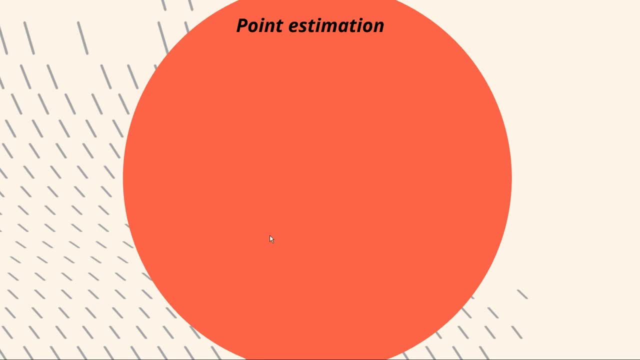 So the final little piece of the puzzle is looking at credible intervals, which is the Bayesian equivalent of confidence intervals. So I've split this particular slide into looking at point estimation and then interval estimation itself. So I guess before we can calculate a credible interval we want to figure out what say 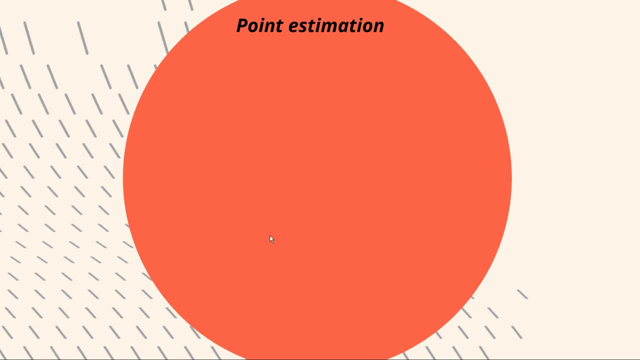 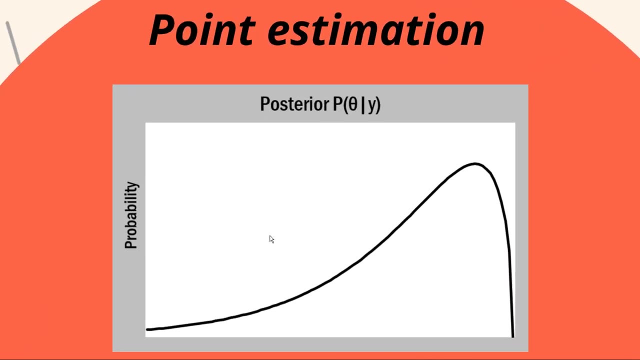 the sample mean or the estimation of our point of interest is. So I've answered this somewhat generally. Here's a particular posterior distribution that happens to be skewed. Now, if you got this as your output- posterior, kind of like the one we got when we were looking- 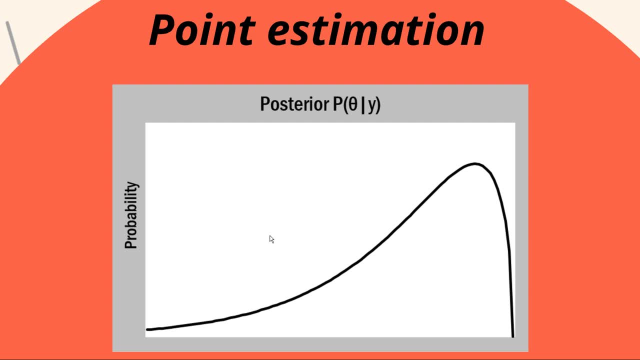 at the coin toss example. it looked a little bit like this: What would be the best estimate you had for theta? Where would you put it? Well, of course, your first instinct might be to say: well, let's put it at the top of this distribution, which is, in fact, the. 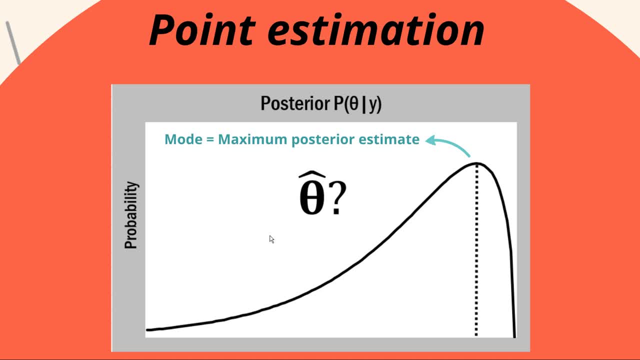 distribution's mode. If you do that, you're going to get the distribution's mode. If you chose to do that, you'll be putting it at the maximum posterior estimate, which would make a lot of sense. But that's not the only possible place to put it. If the posterior 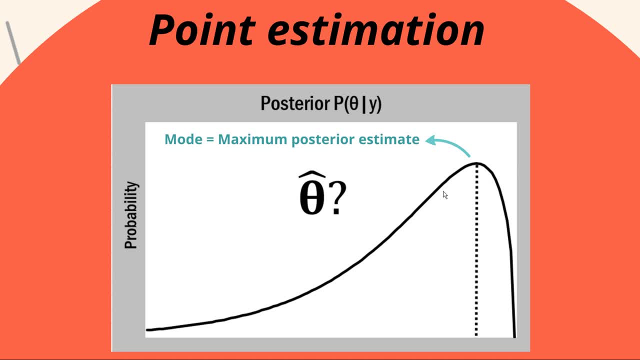 distribution is skewed as it is here. you might want to make it the mean of the distribution, or maybe the median of the distribution, And there may be decent reasons for doing that. The convention tells us to leave it at the mode, but there might be some decent reasons. 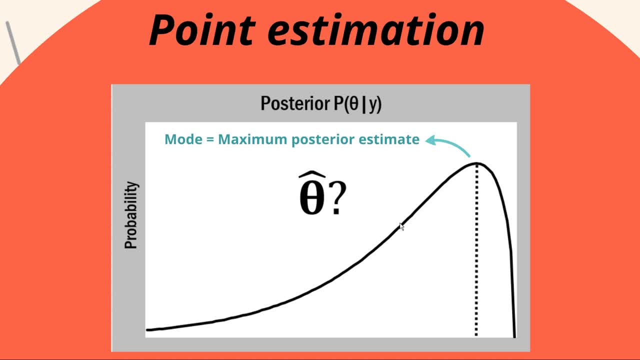 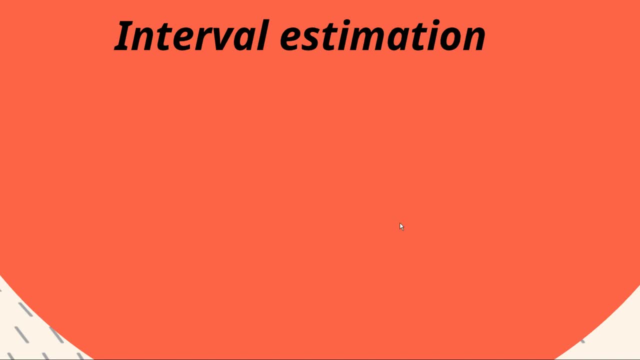 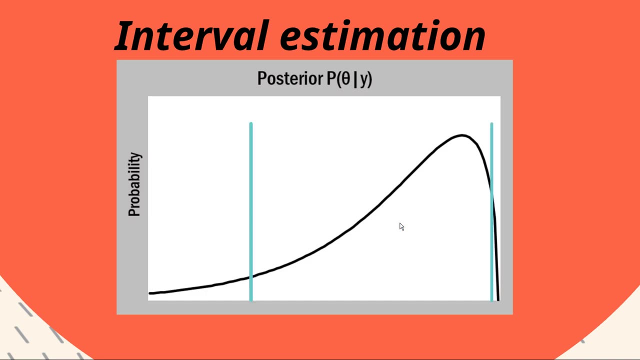 for making it the mean or the median. It's not as necessarily clear as you might have thought. So how then do we construct intervals, So say a 95% credible interval. So if we wanted to much like for frequentist distributions, we can construct a region wherein lies 95% of the distribution. So let's just 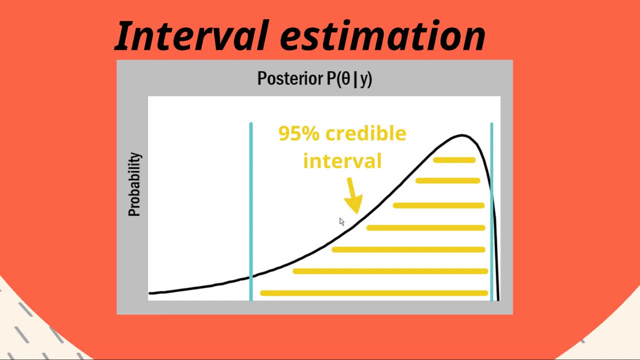 say that yellow region is 95%. Therefore the distance between these two points, the blue lines here, becomes our 95% credible interval. But here's an interesting point to note: I can actually shift these goalposts, I can shift these two blue boundaries and let's just say I don't want to put my credible interval. 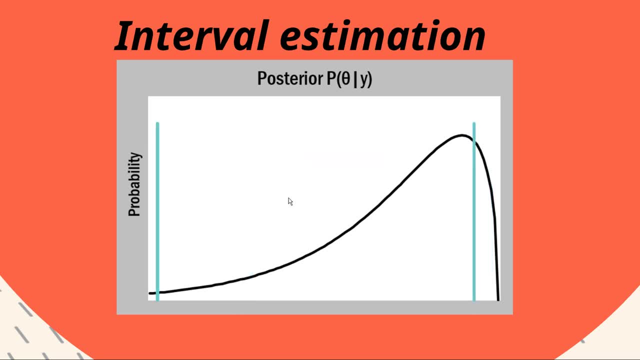 here I can also create another interval, say between these two points, where again there lies 95% of the distribution. So there's not one unique set of boundaries wherein there lies 95%. So we actually need to be a little bit more. 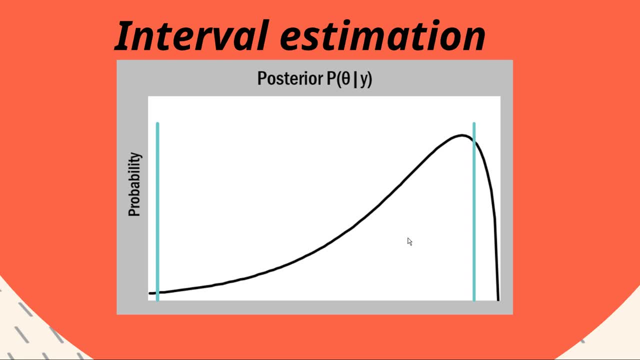 specific if we want to define one credible interval. So often we call the interval the HDI, which is the highest density interval, and it's the particular interval where there's 95% between it. So if I was to color this yellow, there would be 95% in here. but also there is no point. 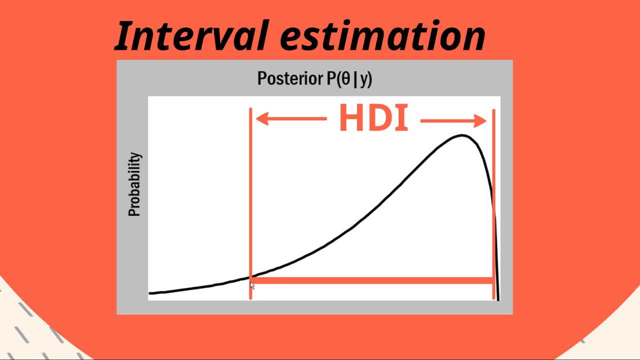 outside of this interval that has a higher probability than the points inside the interval. So if that condition holds, then you know you have the highest, the highest density interval, and that would likely accord with your intuition, at any rate. Now, how do you actually generate these intervals? Well, you're going to need to use some 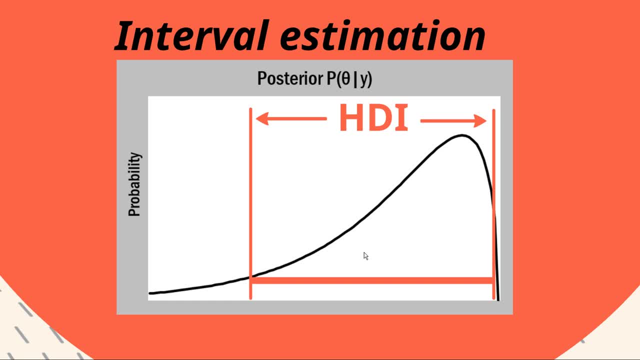 statistical software, so I haven't dealt with in the video here how to calculate your highest density interval. Although keep in mind what happens with your posterior distribution when your sample size gets reasonably large, is that it becomes, is that it approaches a normal distribution. So, even though this is very skewed, this would only really happen with a fairly small 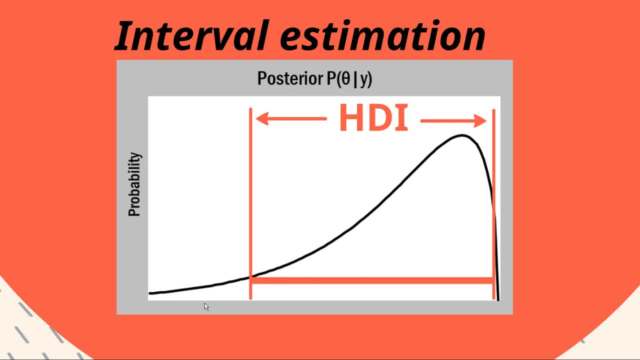 sample. If your sample size increased, much like any kind of sample- everything in the world of statistics- it will approach a normal distribution, at which point you can quite simply construct a 95% credible interval, much like you'd construct a 95% confidence interval. 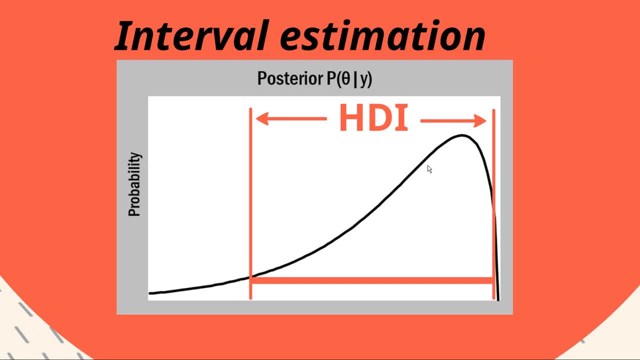 because we know that a normal distribution is symmetrical. so you can start with your sample point estimate and then you can do a 95% confidence interval just using the same formula you would use when you're constructing your 95% confidence interval. so I haven't quite done that for you here, but 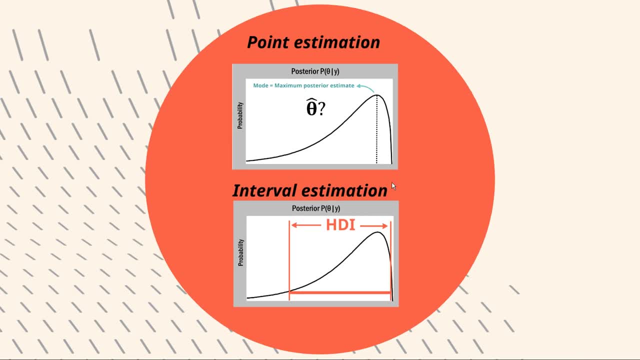 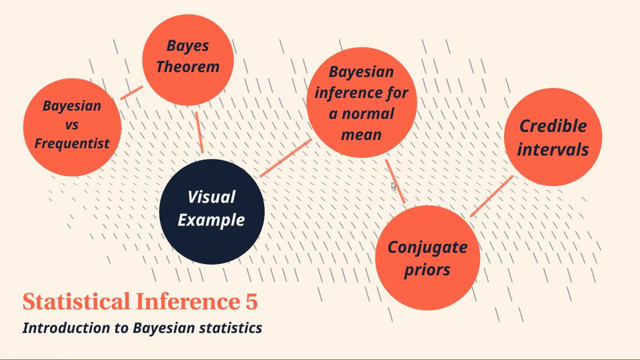 I'm hoping that gives you an appreciation for credible intervals, but then also for Bayesian statistics as a whole. Well, I hope you've enjoyed it. If you like these videos, feel free to have a look at zstatisticscom or the YouTube group Z statistics. I'll put all the social stuff up here and